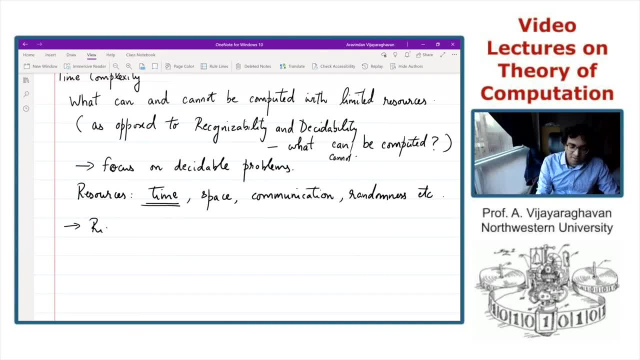 Okay, And this is really a very rich area with many, many challenges and problems that haven't been resolved yet. So there are many open questions And this is really an extremely active area of research. And, yes, there are many big challenges that we still don't understand. Okay, With many. 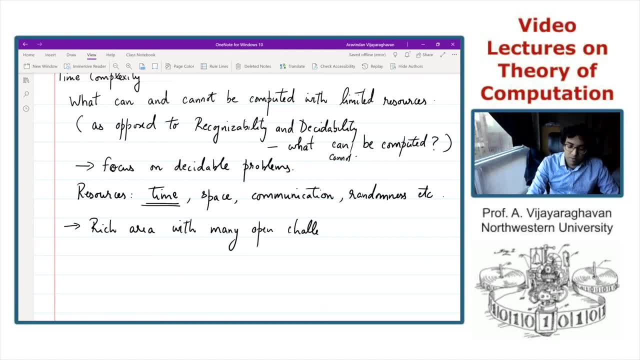 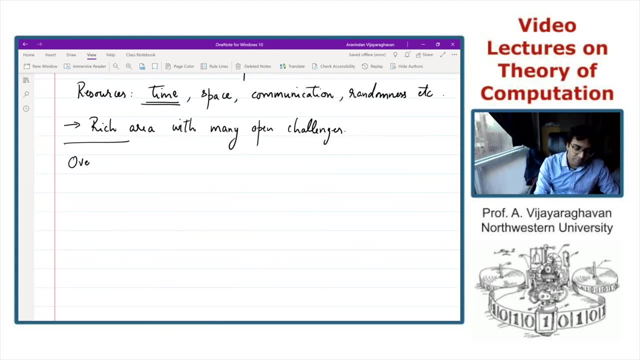 open challenges. Okay, So maybe so for the rest of the lecture. here is the overview. So we'll first define time complexity formally, okay, in the context of Turing machines, And then we'll talk about how you know, we'll talk about these different complexity classes. Let's try to. 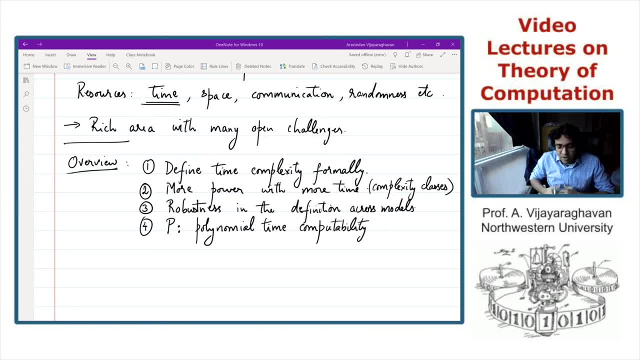 capture a little bit of the concept of time complexity And then we'll talk about how you know it's really telling you how there is more power that comes with more time, So this is really a valuable resource for computation. Then we'll also talk a little bit about the robustness and 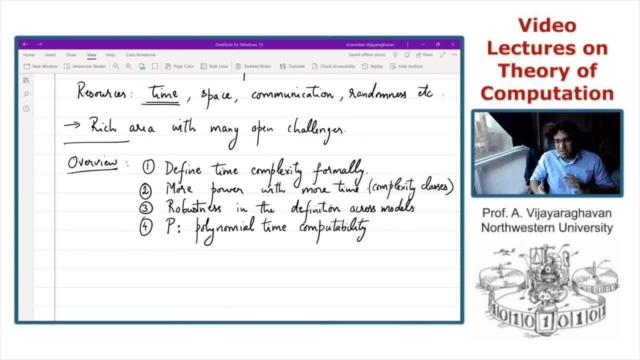 the definition of time complexity across different models. So there may be different models of Turing machines that you can pick, But we'll see that really this notion of time complexity is fairly robust. And finally, we'll talk about the concept of polynomial time computability. 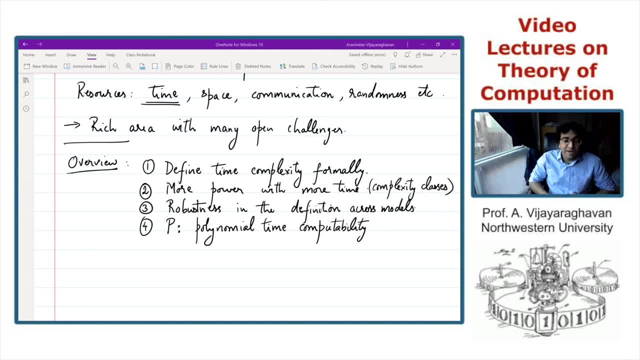 So we'll talk a little bit about the concept of time complexity And then we'll talk about the concept of polynomial time computability. So this is a concept called P, which you may have heard about in other courses, like algorithms, Okay, But this is a central focus of attention in complexity theory. 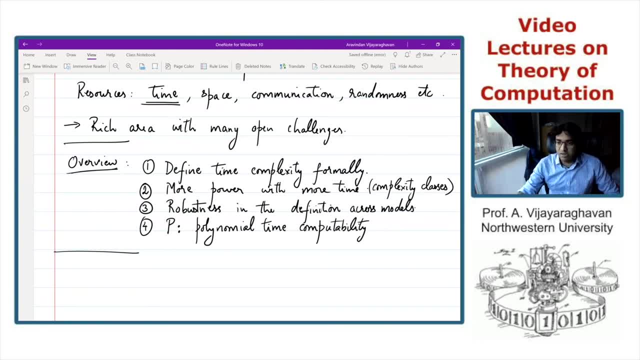 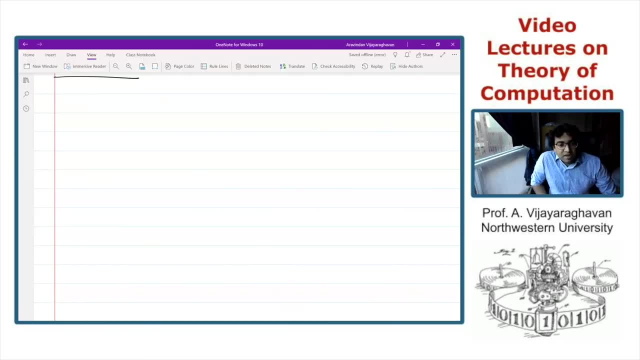 and algorithms. Okay, So this is the plan for the rest of this lecture. Okay, So let's start by talking about, by defining complexity of a time complexity. In particular, we'll be talking about time complexity of a Turing machine first. Okay, So measuring time complexity of a Turing machine. 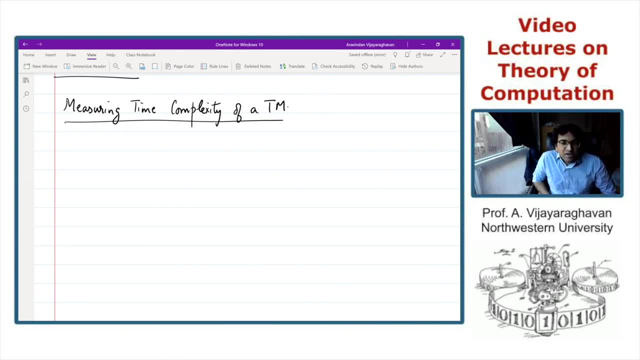 Okay, And really the thing you want to do is you just want to count the number of elementary steps that is required by the machine to halt. Okay, So let M be a Turing machine that halts on all inputs. Okay, And remember, we are only focusing on decidable problems, So 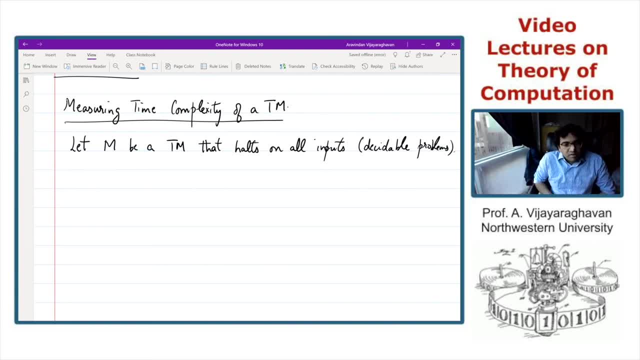 okay, So let's think about a Turing machine that halts on all inputs. Okay, Now the time. complexity will be measured in terms of the input. Okay, In particular the size of the input. Now, the size of the input can actually depend a lot on the problem. So there, 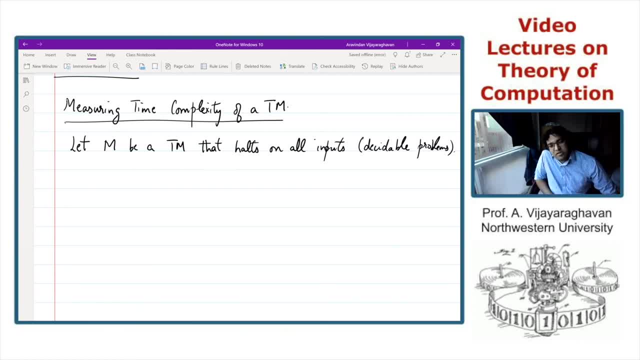 may be various parameters for a problem. For instance, if you think about a graph problem, then different parameters could be the number of vertices, or the number of edges, or the degree of the graph, and so on and so forth. Okay, Okay, Okay. 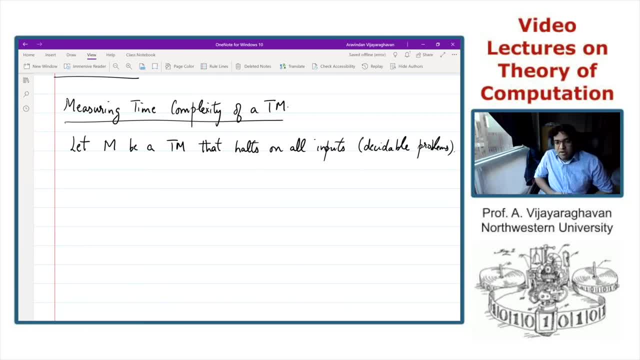 Okay, Okay, Okay. What we'll do in this lecture and throughout this course is we'll just focus on, we'll use the size of the description of the input as just the input size. Okay, So the input size is just going to be the size of the. 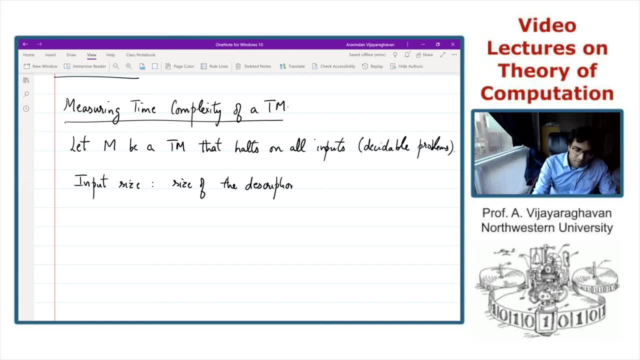 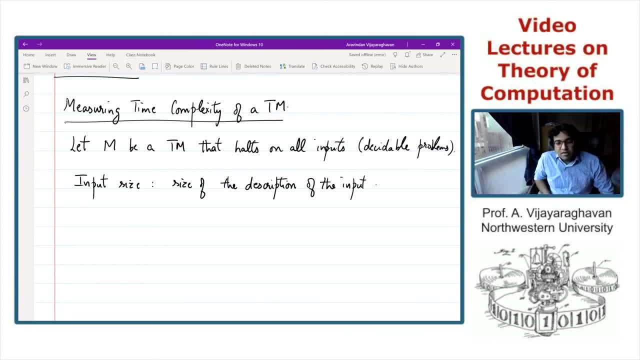 Okay, And this is really what we're going to do. This is consistent with what we do with Turing machines. So we just think of the input as being a string, okay, over some alphabet, let's say 0,, 1.. And really the size of the input is just the length. 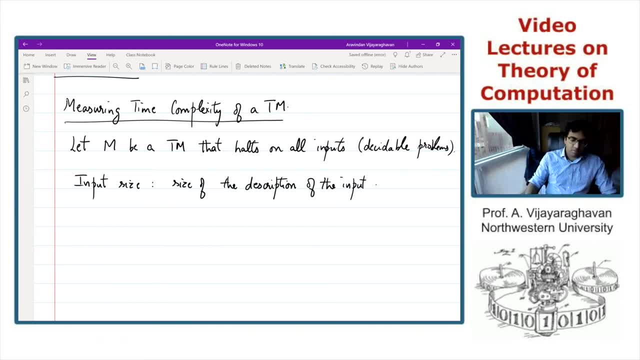 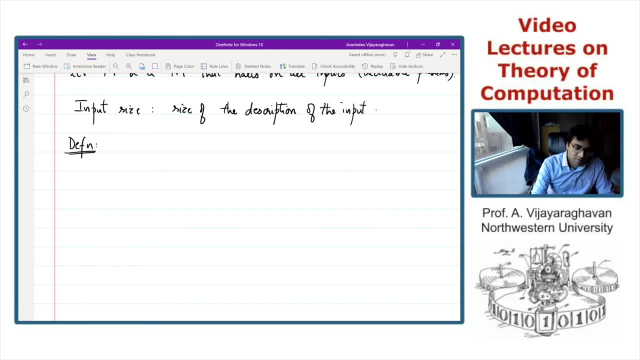 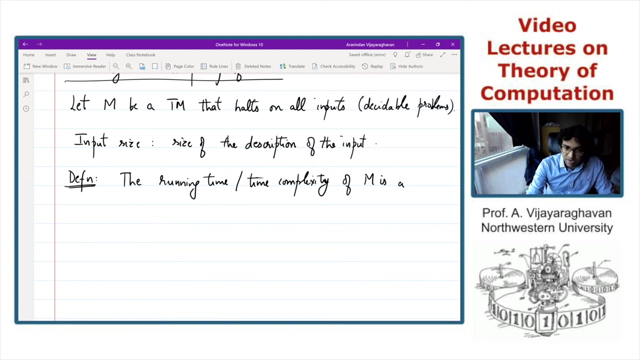 of the string that represents that input. Okay, So here is the definition of time complexity. Okay, So the running time, or time complexity, or time complexity or time complexity of the Turing machine M is really a function. Okay, It's not a number, it's a function which depends on the input size. 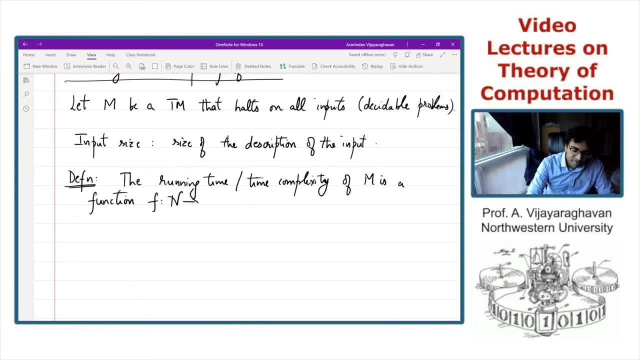 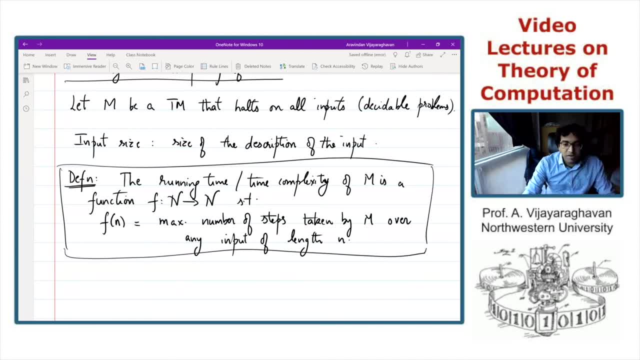 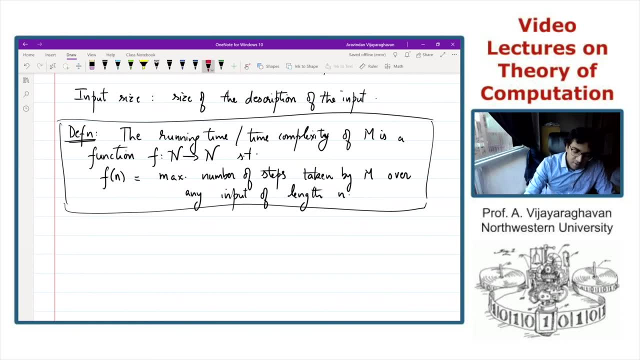 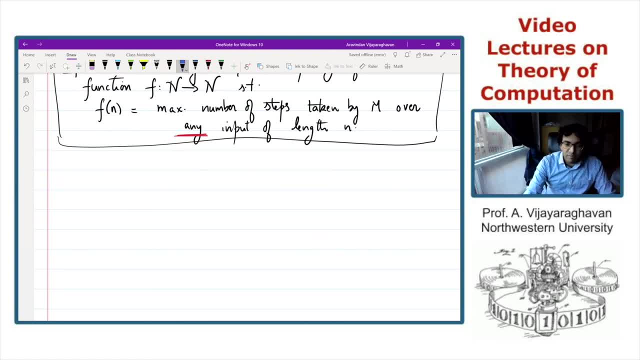 look over all the possible inputs of length n and f is actually going to be the worst among all those inputs. So this is really a notion of worst case analysis. Okay, So this is the definition of the time complexity of a Turing machine. Okay, So one thing that's important to note here is that is to focus on any. Okay, So we are going to look over all the possible inputs of length n and f is actually going to be the worst among all those inputs. So this is really a notion of worst case analysis. 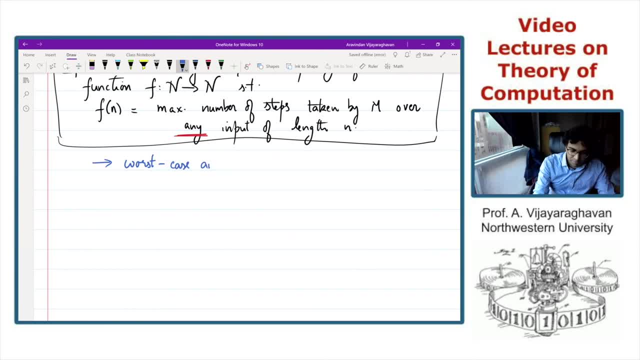 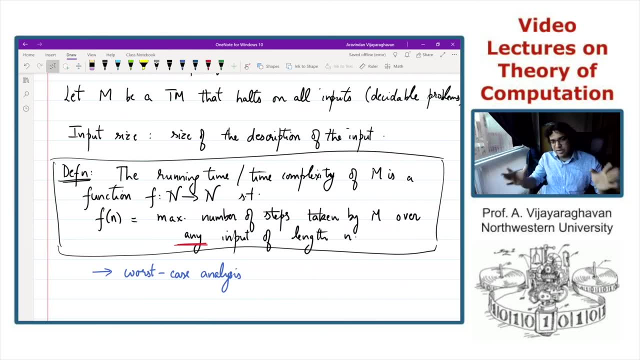 Okay, So this is really a notion of worst case analysis. Okay, So for a Turing machine M you look at, I mean, and for a particular input, size small n, you look at all possible inputs of n of size n and f is exactly the time. complexity, 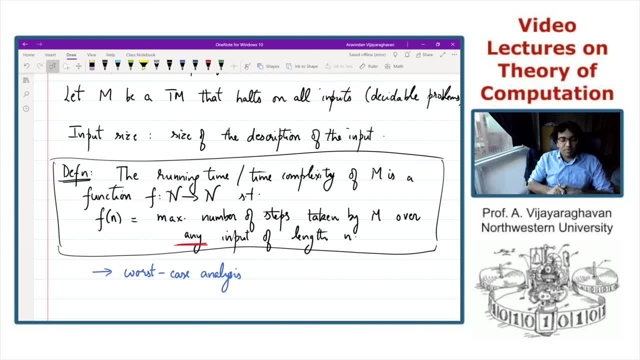 of n is just going to be the maximum number of steps that the Turing machine takes, Okay, Over all possible inputs of size n. So this is the worst case notion of complexity, And this is what we'll traditionally use, And this is what is traditionally used in computer science, in theoretical computer science. 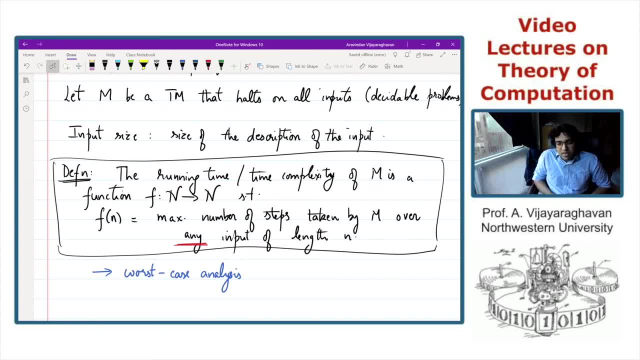 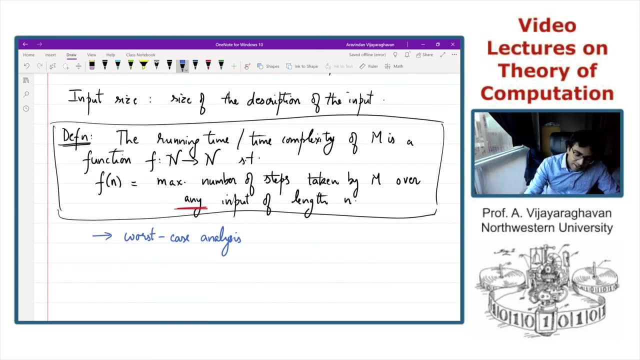 Of course, there are other notions that are used as well. That could be an average case notion of complexity, And there are things that go beyond worst case analysis, but that is out of the scope of this course. Okay, And the second point I'd make is that 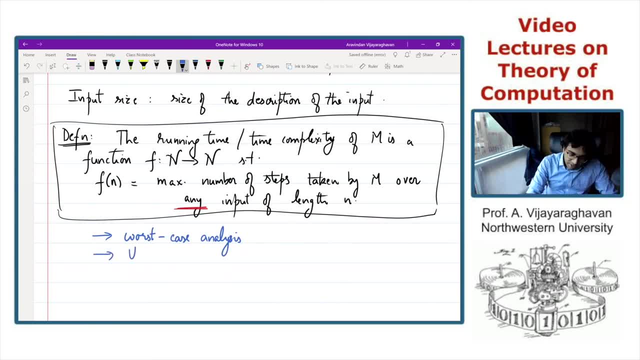 here. when we talk about time complexity, we'll predominantly use the big O notation. Okay, And this is consistent with how you analyze algorithms as well. Similarly, when you're talking about the time complexity of a Turing machine, use the big O notation, And this is something that I would. this is something that's covered. 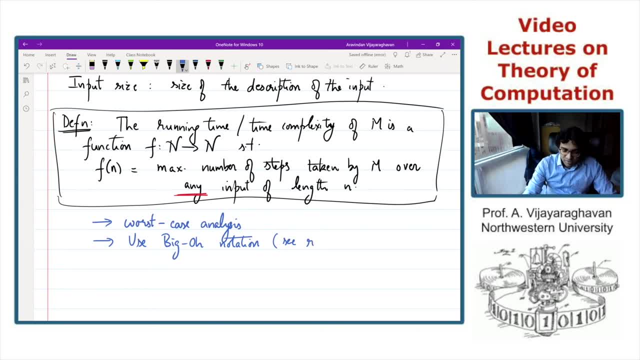 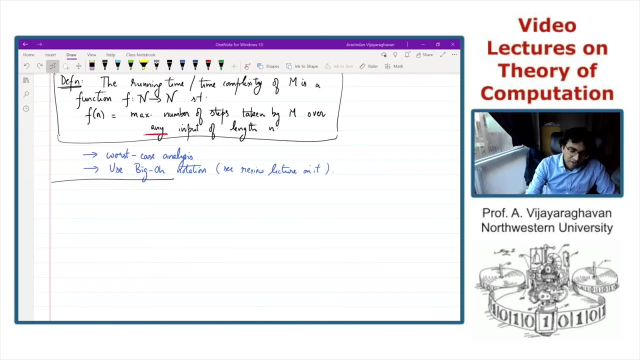 in one of the review lectures. Okay, So see review lecture about it. if you have any questions, Take care. Okay, so this is the time. complexity of a Turing machine. Now let's look at an example. Okay, And let's look at this language that we had considered before, which is: 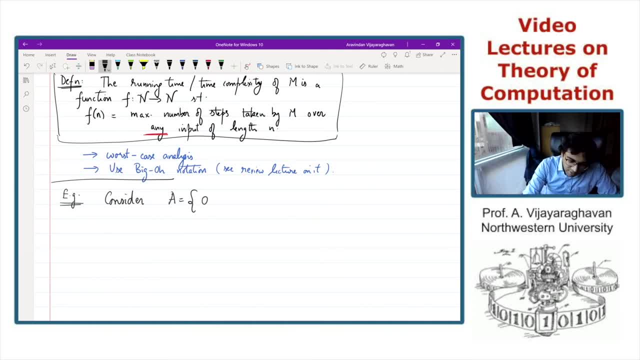 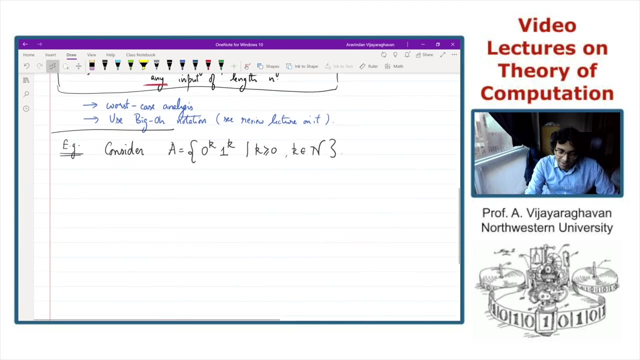 the set of all strings consisting of zeros, and ones where you have a set of zeros followed by an equal number of ones. Okay, Ok, Ok, yeah, I mean, of course, k is a natural number here. Okay, and remember, this was a language. 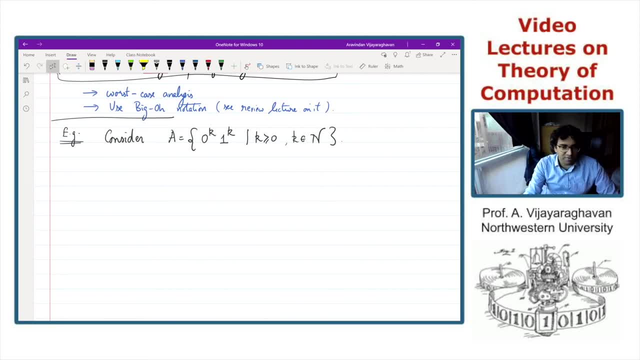 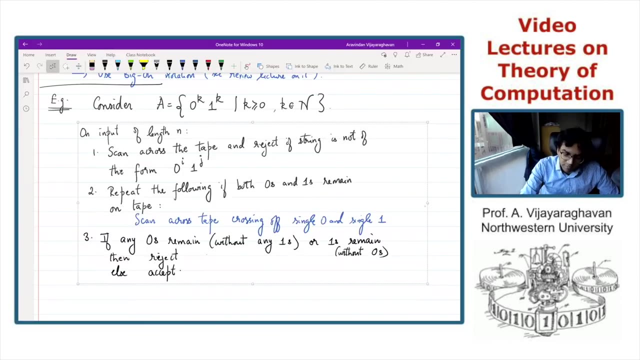 that was not regular. however, you could construct a Turing machine for this task. Okay, now here's a simple Turing machine that implements this, that recognizes this language, in fact, decides this language, In fact. here is a pseudocode that represents this Turing machine. So, on an input of size n, let me just- I just copied it just to save some time- on an input of: 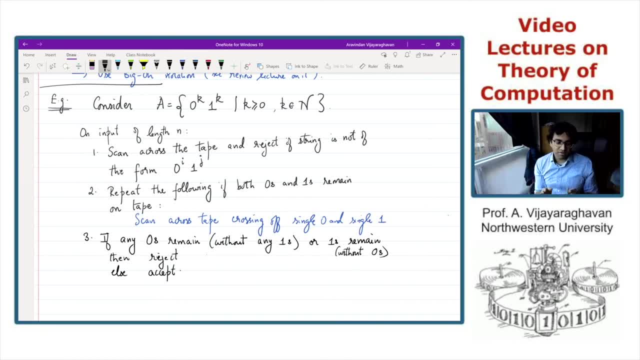 size n. what the Turing machine does is you just scan across the tape first. okay, do one scan of the input to ensure that the input is just consisting of a string of zeros followed by a string of ones. Okay, here you're not checking if the number of zeros and ones are equal, you just 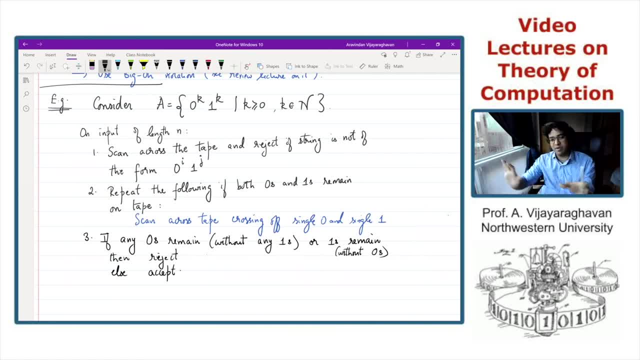 want to see that it is of the form: some zero, a bunch of zeros followed by a bunch of ones. and that's the first step, Okay, and the second step is to basically repeat the following: where you know you go from across the tape and you, you kind of cross off a single zero followed by, and then you go across the tape. 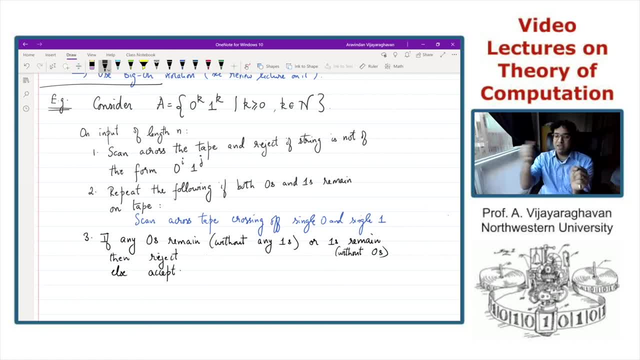 to where the one start, and then you cross off another one, Okay, and then you come back, cross off yet another zero, and then you go and cross off an uncrossed one, and so on. Okay, you just keep doing this. Okay, and this is the Turing machine that we've seen before, and and then 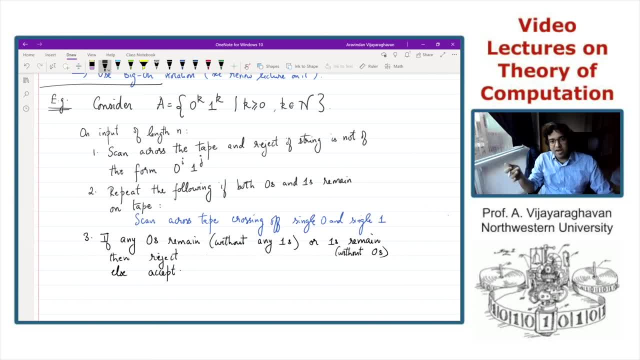 finally, if any zeros remain uncrossed, and but all the ones have been crossed, okay, or if there are ones remaining and all the zeros have been crossed, then you reject. Otherwise, you know, none of the zeros or the ones are left and crossed, in which case you accept. Okay, this is the Turing machine. 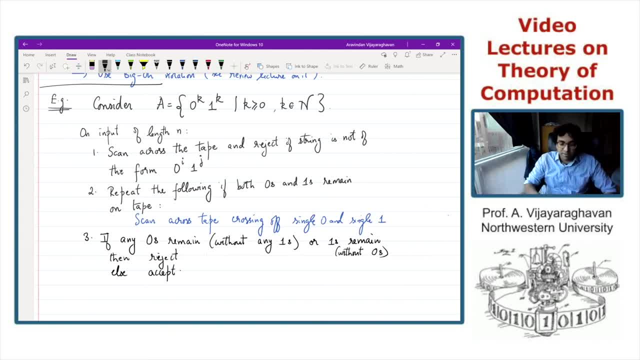 that we've seen before. Let's just analyze the time complexity of the steering machine. Okay, well, the first step is, I mean, so we, we stand across the tape just to check if it is of the form a bunch of zeros, followed by a bunch of ones, and this one second. 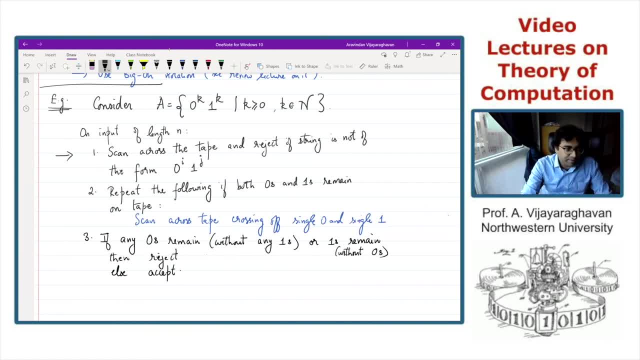 Okay, so let's just continue writing. So this step takes time, which is all the way to the of n, because the input is size n and it just, you know, scans. it's just one scan across the input. Now the next step is a little more interesting. okay, because you keep going off and crossing. 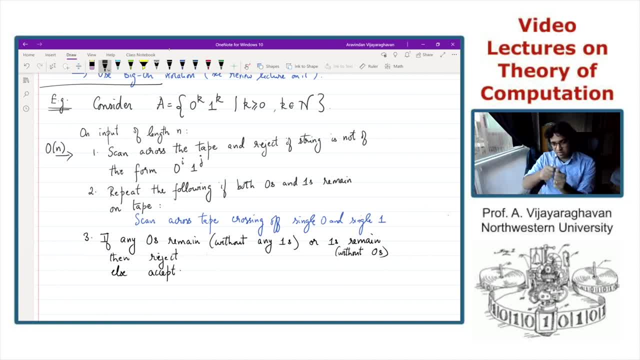 off one zero and then followed by crossing off a one, where you go across the tape and then you come back and cross off another zero and then you again go across the tape to to cross a one. and so each time you cross off a zero and a corresponding one you may have to. 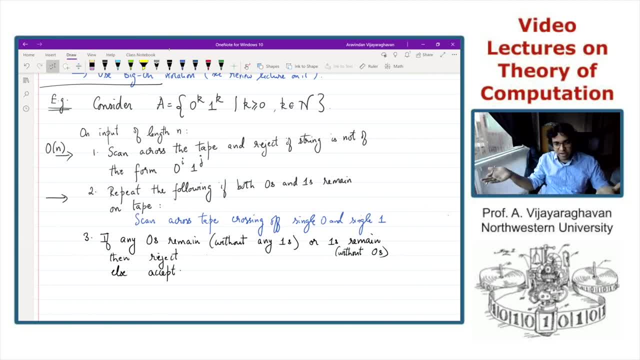 go across almost the whole tape. so that's an order n step. but that's for crossing of one zero and one one. okay, but you have to do this for roughly n over two zeros, so okay, and then over to one. so this is an order n squared operation, okay. Then finally, 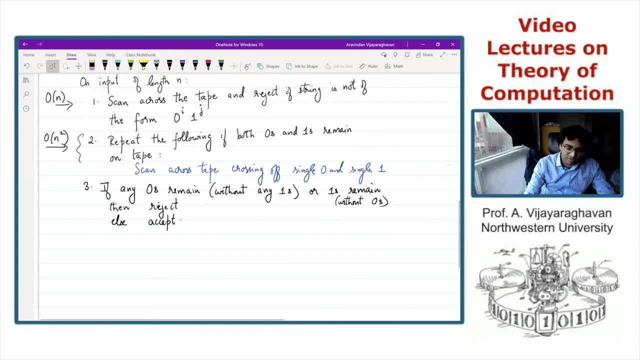 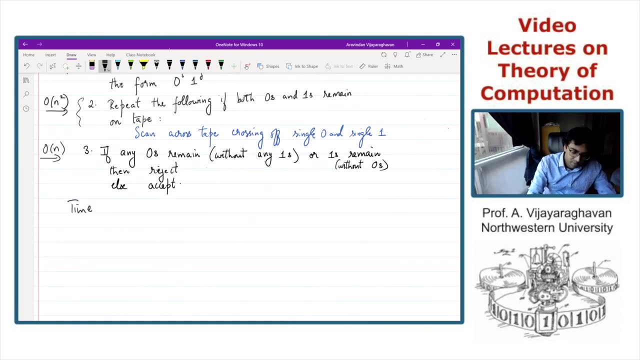 are you just going to check if there is any zeros remaining or ones remaining? and again, this is potentially, and you just need to do one scan of the tape. this is an order n operation. Okay, so the time complexity of the steering machine, remember, is the worst over all possible inputs. okay, and 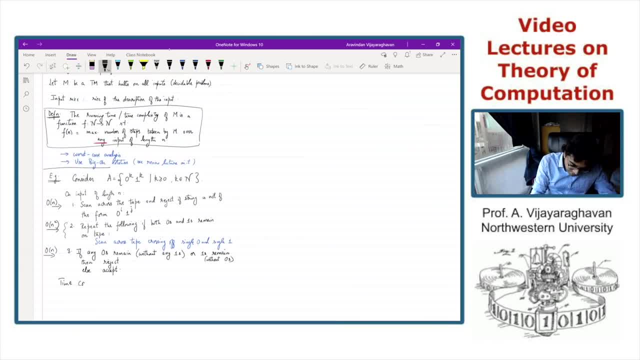 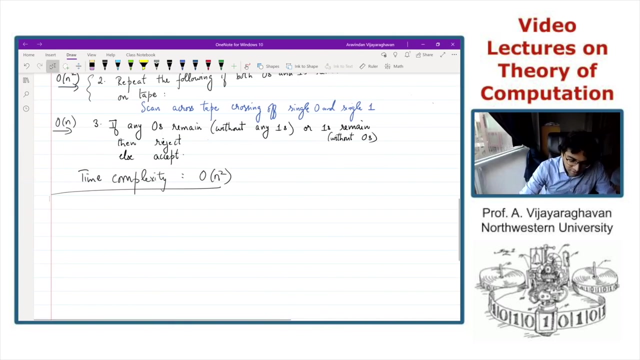 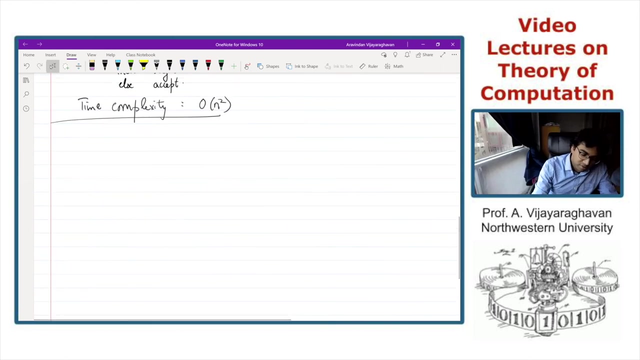 of the time it takes on input n and the time complexity is. hence order n squared, okay, good, okay, so that was the time complexity of a single turing machine. okay, but now let's try to extend this concept from, i mean, particular turing machines to languages, okay, so, so we'll see the idea of 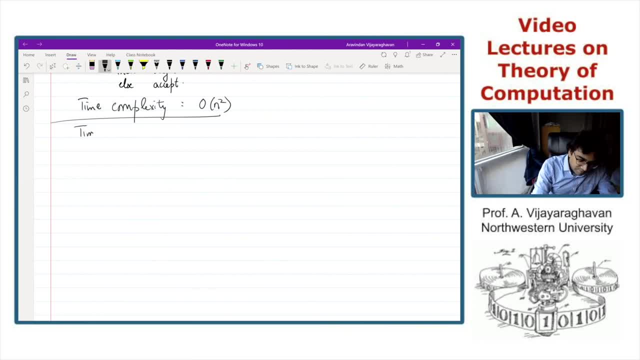 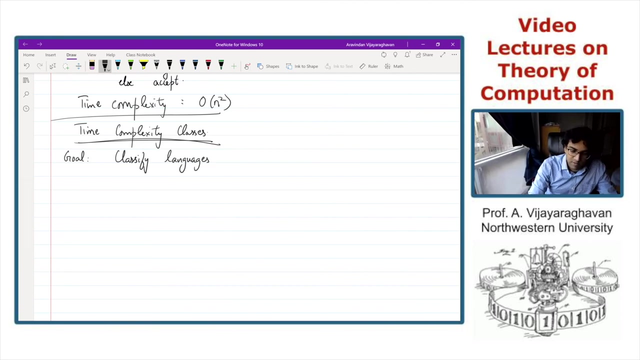 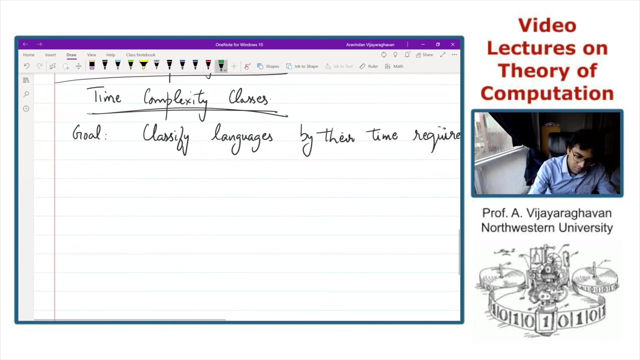 this leads us to the idea of time complexity classes. so the goal is to classify languages okay, by their time requirements. so this is the time sector in this엔. okay, the class. so think of t of n as just a function of n. so the time, the class, given by time, of this function, t of n, okay, um is really the set of all languages. 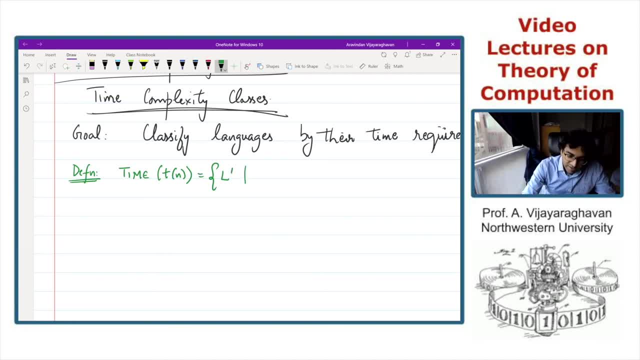 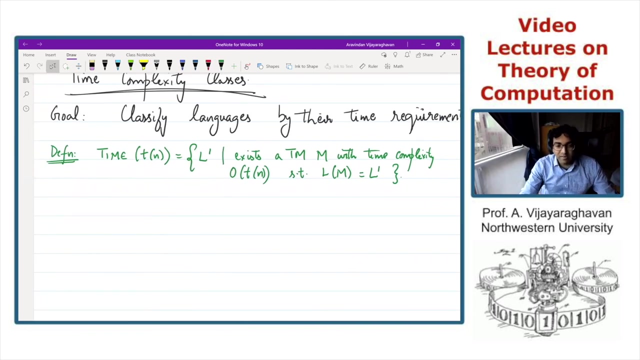 l prime okay, such that there exists a turing machine, okay m, with time complexity order t of n l, which actually accepts this language. so l of m should be equal to l prime okay, so. so one thing that's important to note here is that this consists of all languages. 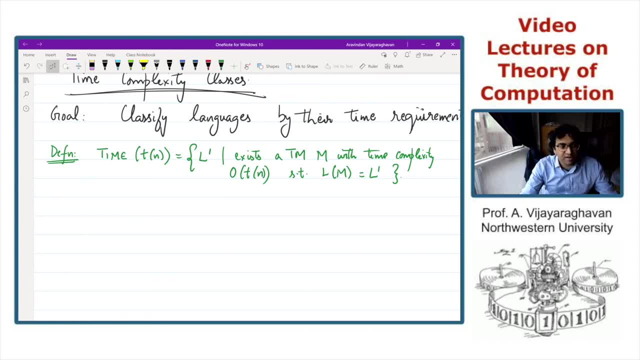 just of all languages, just so. one thing that's important to note here is that this consists of all languages for which there exists a Turing machine, which has complexity at most order t of n. So there might be Turing machines for this language. that could take actually more time. 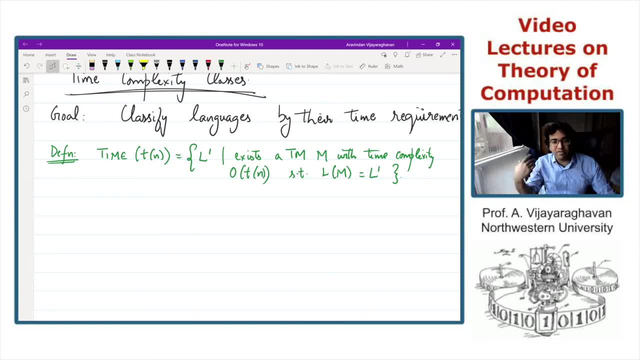 But for, among all the Turing machines that accept this language, you can choose the minimum, the one that has the least time requirement, And then if its time requirement is given by the function t of n, then this language is in time of t of n. So, for example, 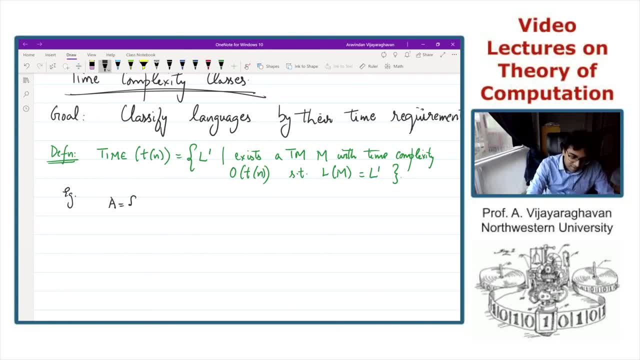 this language, A that we looked at, which was given by strings of zeros and ones where you have zeros for a bunch of zeros followed by an equal number of ones. this language is given by earnings of t of n raised to the time of t of n. 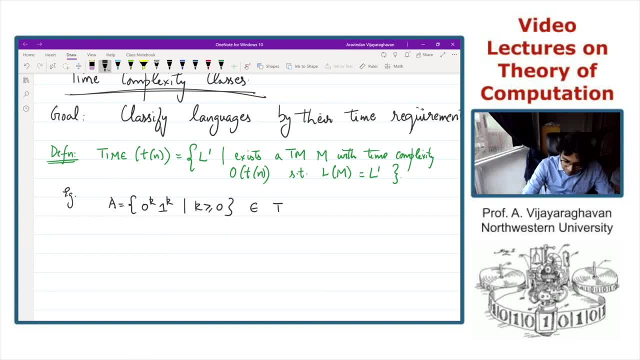 It's sometimes the story of TI. So your theorem is as simple as giving a function this for, consequently the t of n, then language we just proved- is in time n squared. okay, so here t of n is the function n squared. okay, now, because this is in time n squared, it is also in time. 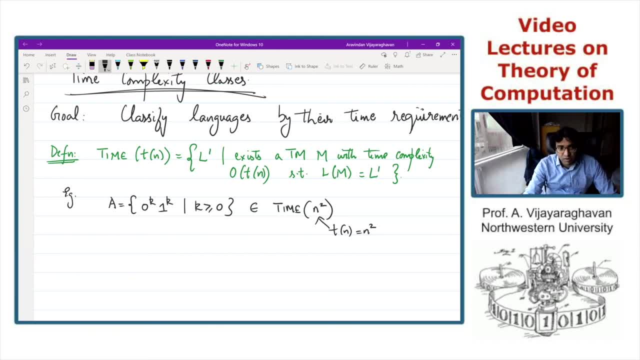 n cube or n to the 4 or any larger function than n squared, because, uh, note a is also in time n cube or anything else. okay, anything higher, because this is still, since n squared is still order of n cube. okay, according to the big O notation. okay, um, so it is certainly in a. 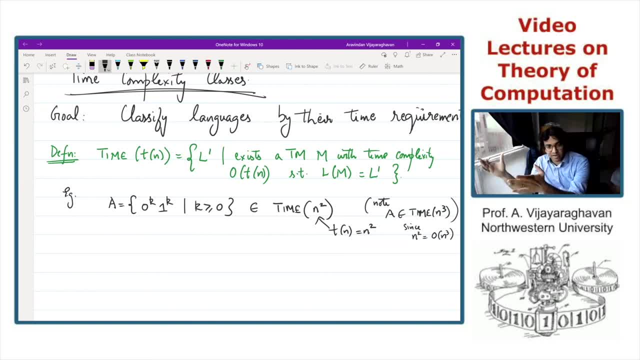 it is certainly in in a larger time complexity class. so it is certainly in a larger time complexity class. it is certainly in a larger time complexity class. but typically you want to show, you want to find the smallest function t of n for which the language actually, I mean where the language decides. 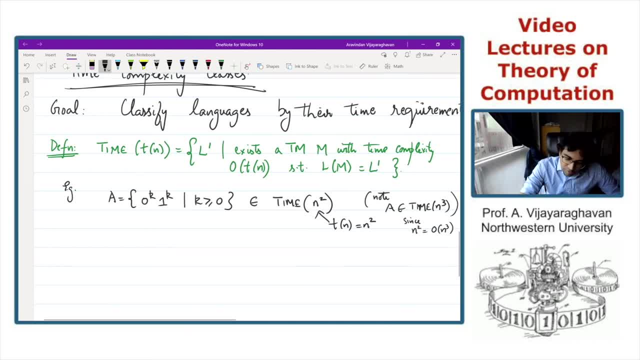 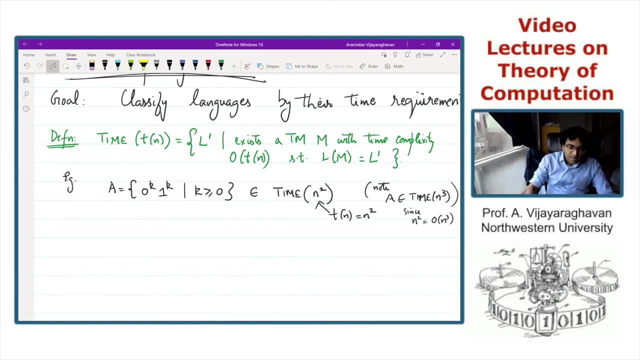 okay, so good. so this is a notion of, I mean, this is time bounded complexity class. okay, sometimes this is also referred to as I mean referred to by you know d time, d of n. this is just an alternate notation, okay, and we will see why a little later. 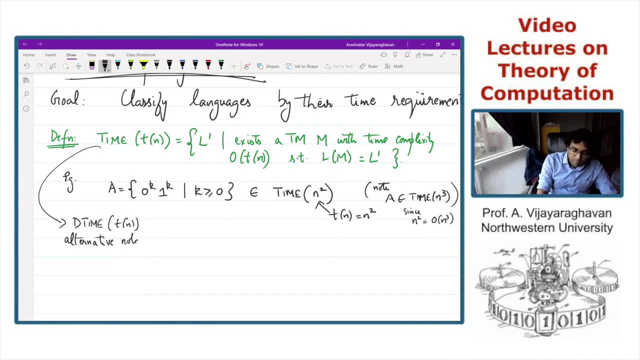 okay, this just stands for deterministic time. good, okay. so now we know that the the class a resides in a time of n squared in the class time of n squared. okay, But it perhaps also resides in a time complexity class which corresponds to the smaller time requirement. 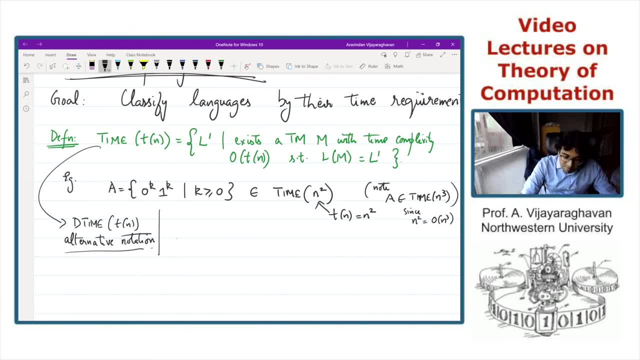 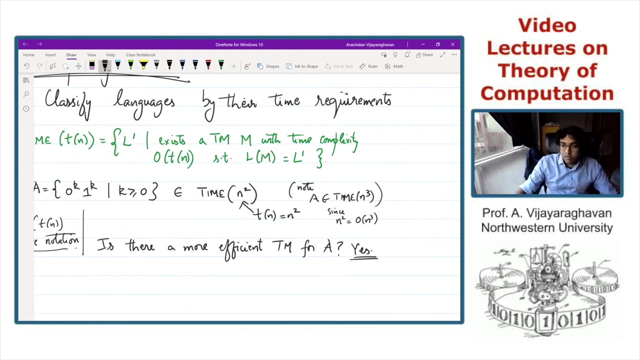 For instance. I mean. so the real question is: maybe there exists a more efficient tuning machine for A? And it turns out that the answer is yes, You can actually do something more efficient, more interesting, And we'll just see this. 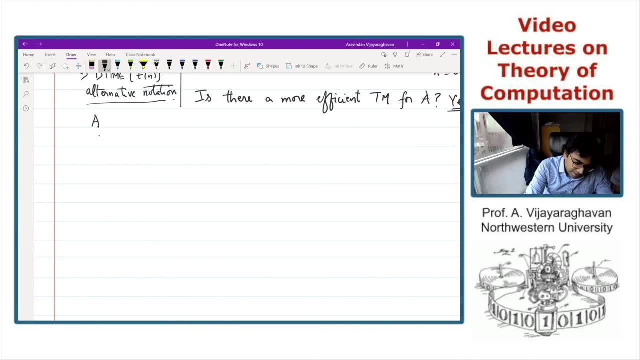 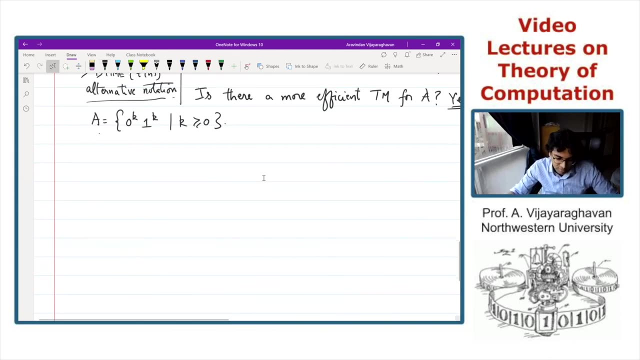 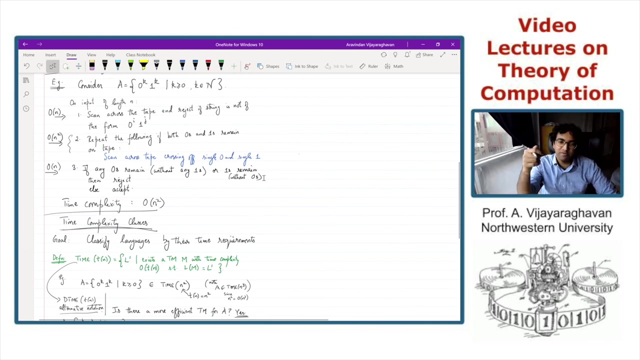 So we call that. A is the language given by 0 to the k, 1 to the k. k is a natural number greater than or equal to 0. So actually so we saw a tuning machine before for this, which is basically scan through the input and then crossed off. 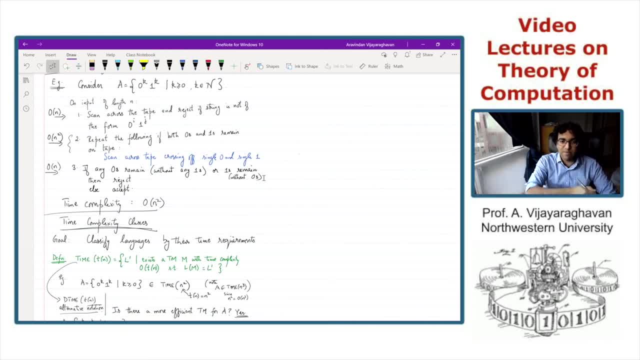 For every 0,. you went and crossed off a 1, and then came back, crossed off another 0, and then crossed off another 1.. But you can try to be more efficient about this: When you cross off a 0 and you go and cross off. 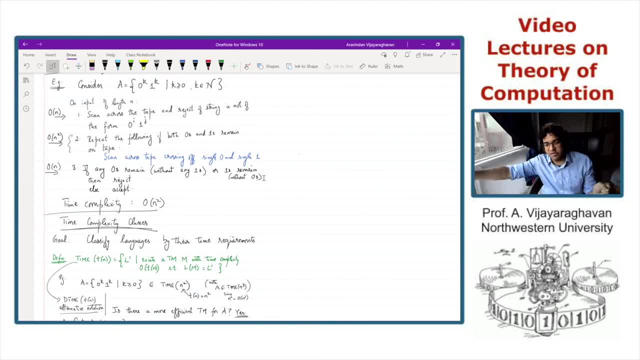 a corresponding 1,. you have to go all across all the other 0s and then, before you go and cross off a 1.. But maybe if you can cross off multiple 0s at a time, then you can be more efficient. 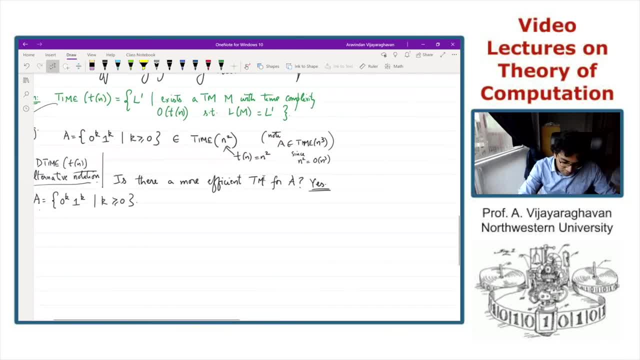 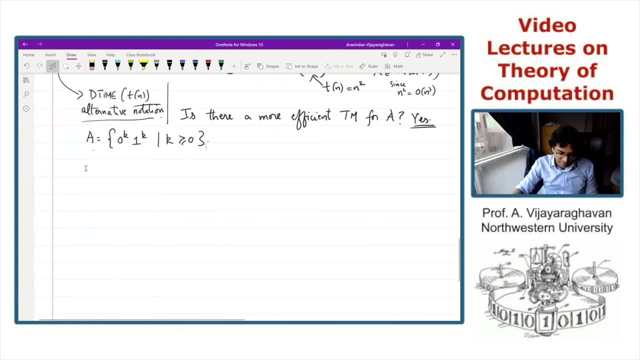 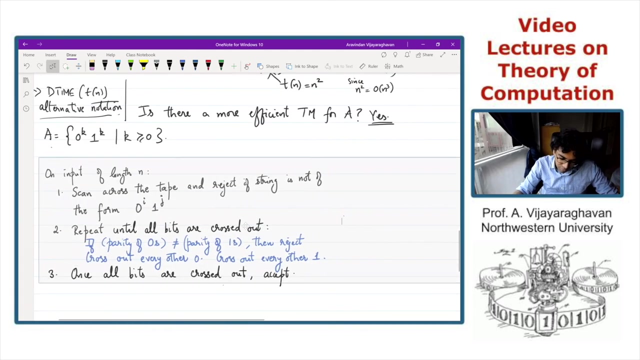 And this is what the algorithm will actually do. So let me actually show the pseudocode for it And, in the interest of time, let me just paste the pseudocode for it. So this is the algorithm. So, as before, the first step is to just scan. 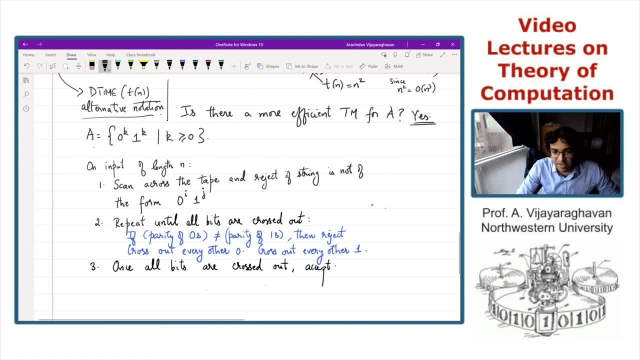 through the input And check that the string is actually of this form: 0 to some bunch of 0s, followed by a bunch of 1s. OK, But now it's going to do something more interesting. OK, First you check if the parity of the number of 0s 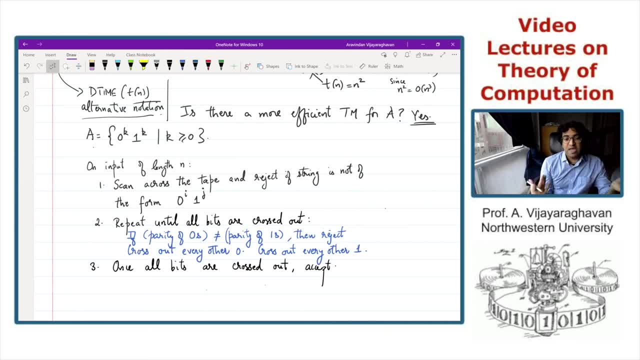 is equal to the parity of the number of 1s. If it is not equal, you just reject the string. So for instance, if you have �, you're going to say, you have you know 10 zeros and 13 ones then the parity of 10 which is i mean even is not equal 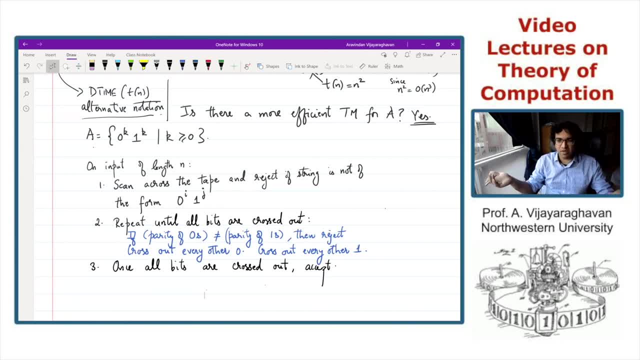 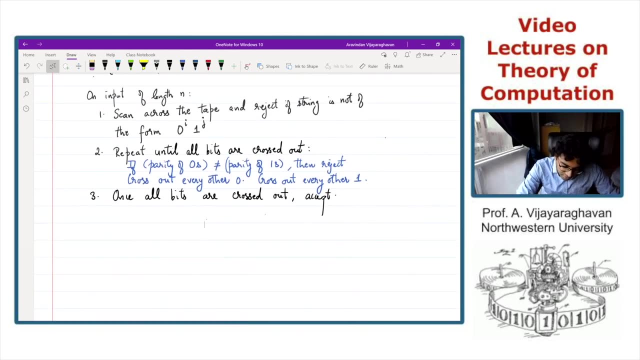 to the parity of 13, and so you just reject. on the other hand, if, uh, you know it has 10 zeros and 12 ones, you're not going to reject at this step because the parity is both even okay. so this is just a check that you do, okay. and then here's where you do something more interesting: uh, you. 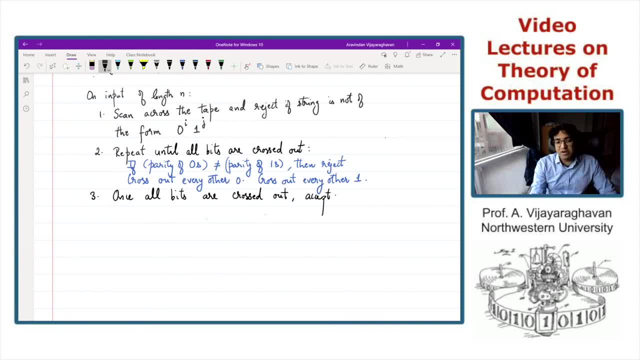 basically cross out every other zero. you're not crossing out just one zero and then going and looking for its partner one. you cross out every other zero, every alternate zero, and then you go to the ones and you again cross out every other one. okay, and then you basically kind of keep. 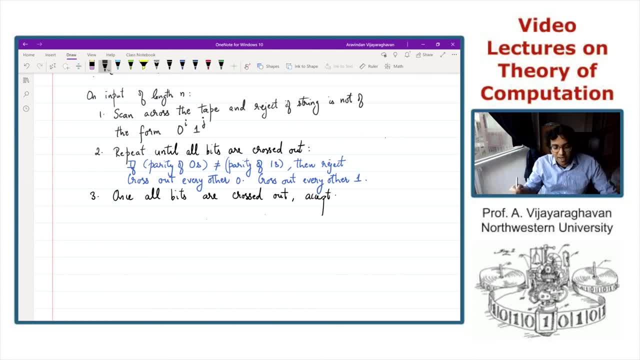 repeating this. okay, so you, you do this and then you go back and you check if all the bits have been zeroed out, okay, and, uh, you know, you check if the pattern is the same. please take a look at here. that's nothing to worry about here. and then the first step is theвод. is that okay? wow, so i has. 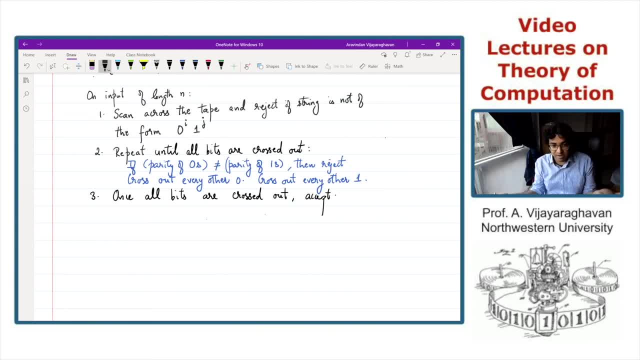 parities of the zeros. the remaining zeros is equal to the parities of the remaining ones or not. if they're not equal, you reject, otherwise you go ahead. and then you keep doing this until all the bits have been crossed out, and at the end of it, when all bits have been crossed out, you exit. 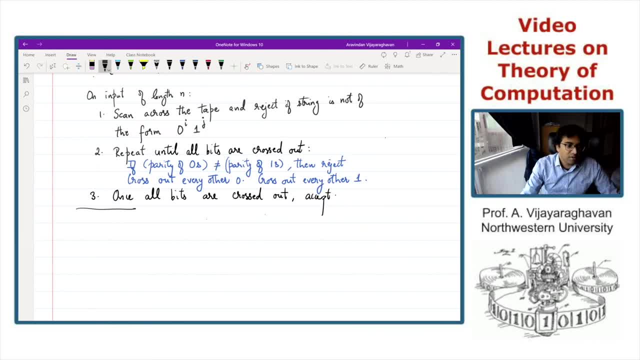 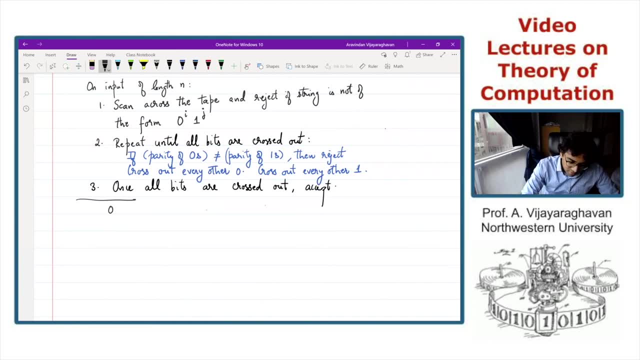 okay, good, so let's see an example. okay, so that, just to make things a little clearer. okay, so, let's look at a string where maybe there are eight zeros and eight ones. okay, so, this is something that is in the language. again, recall that. okay, this is in the language. 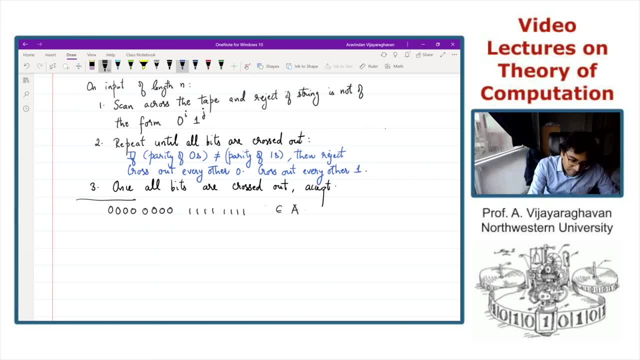 now, what does the algorithm do? it scans across the tape and first, you know, you check that the parity is the same, okay, second, let me just get the one of these different colored markers. good now, you just first change the variety of the parity and then you check that the parity is the same. 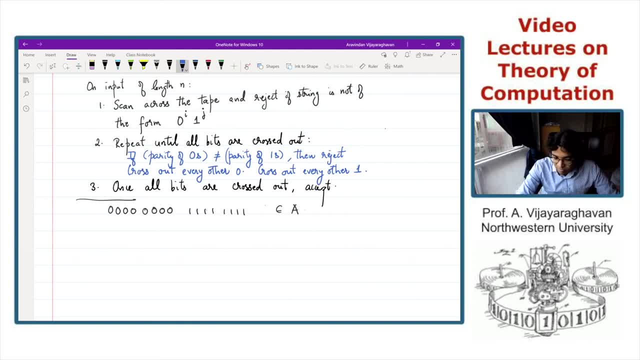 check that the parity is the same for the zeros and the ones, and they're both equal. in fact, they're both equal to eight. so if the number of zeros is actually equal to the number of ones, you will always be fine in that step. okay, and now what you do is you go and strike out alternate zeros. so 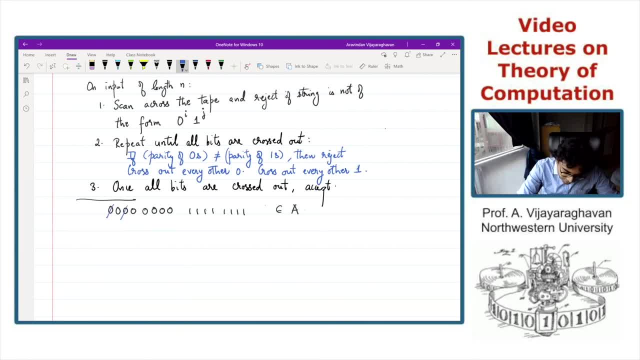 you start, you cross out the first zero, then the third zero, then the fifth zero, seven zero. similarly, you cross out alternate ones: the first one, the third one, the fifth one and the seventh. okay, now go back and check if- okay, i mean, there are still some zeros and ones to be crossed out. 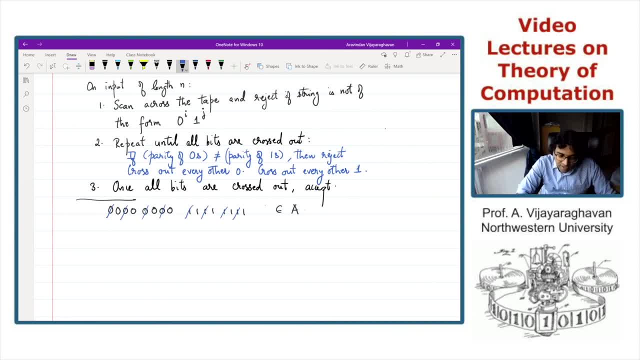 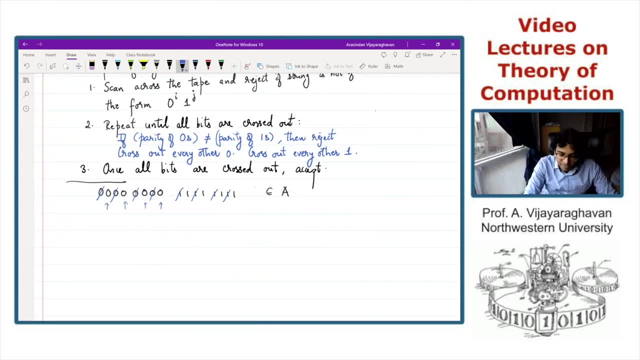 and then you check if the parity of the remaining zeros and the remaining zeros is four of them. okay, so so it's this one, this one, this one and this one. there are four zeros left and exactly four ones left, so the parity is still the same. okay, now you go in and you start crossing. 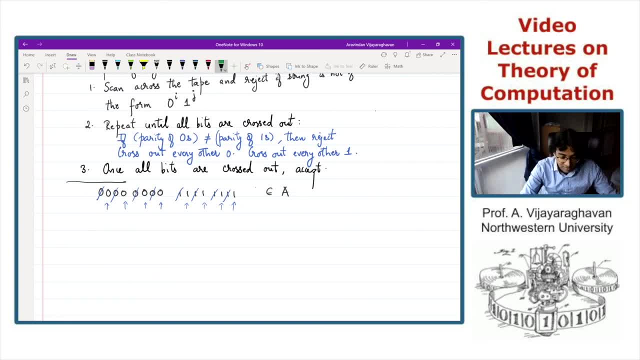 out again alternate zeros among the remaining ones that are left. so you cross out the first zero remaining zero left. you will not cross out the next remaining zero left. again. cross out, okay, the third remaining zero and leave the fourth one. similarly for the ones, cross out the first one remaining and then the third one, okay. so now how many zeros are left? this one is: 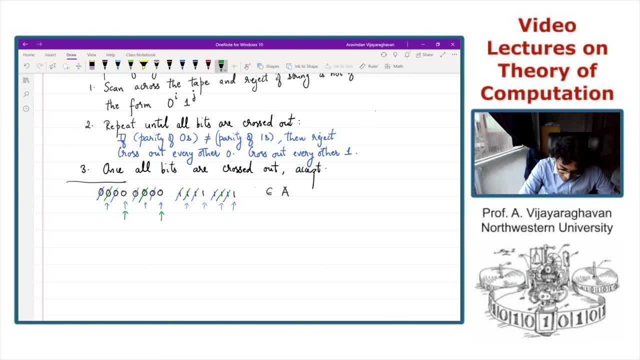 left and this one is left. similarly, among the ones, this one is left and this one is left. again, the parity is the same. you continue and you cross out maybe another. cross out the first zero, leave out the second one. similarly, because of the first one, leave out the second one. okay, again, the parity will. 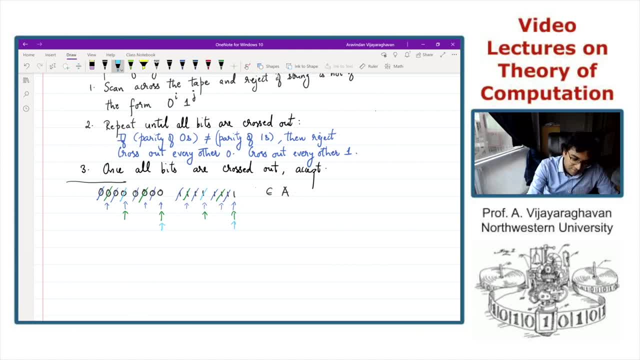 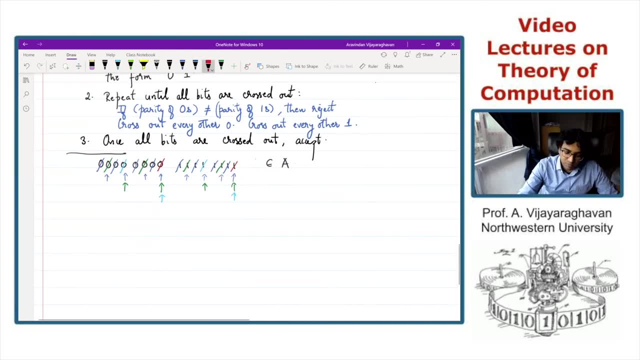 remain the same. this is left, and this is left, and finally, we cross out this one and this one, and now all of them have been crossed out. so so, this is in the language. on the other hand, And if it had been a different number of zeros, 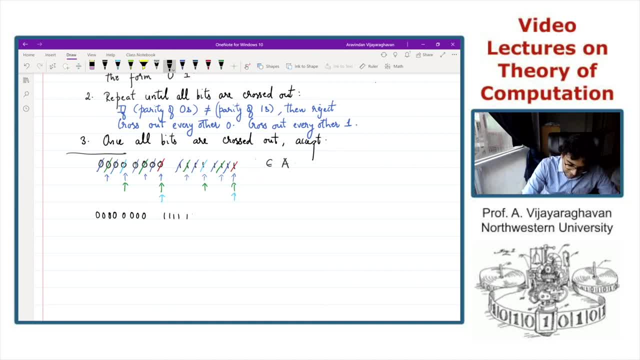 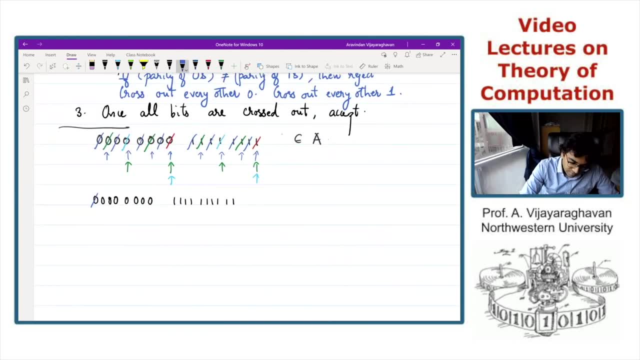 okay, one, let's try it with five, sorry, 10 ones. Okay, in the first step you cross out the alternate zeros, So this will cross out all of these and then cross out alternate ones. Okay, so now the remaining ones have how many of them? 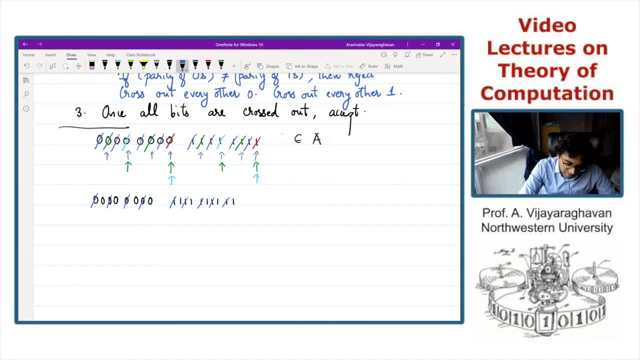 There are four of these zeros and how many ones are left? One, two, three, four and five. So the parity is not equal at this step, because there are odd number of zeros left and even number of ones left. So this is not an even number of zeros. 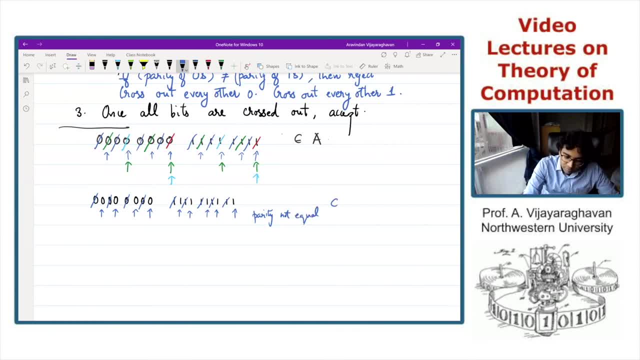 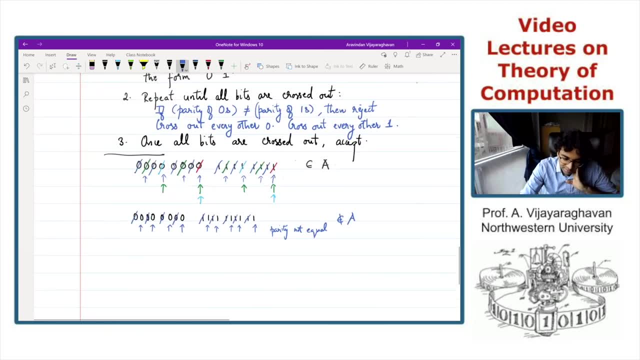 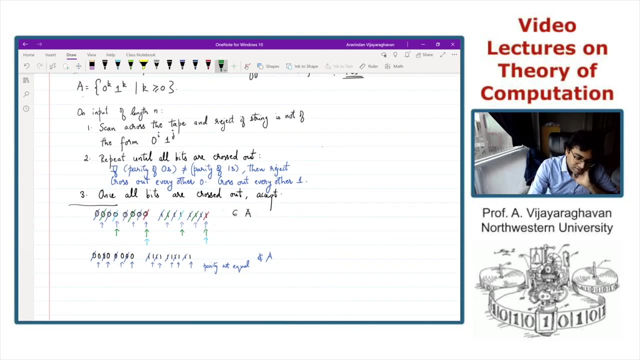 So this is not an even number of zeros. Okay, so this is the algorithm. Okay, good, and what is the time? complexity of the algorithm. Well, the first step is still gonna take order and time, because it's just doing a scan across the whole tape. 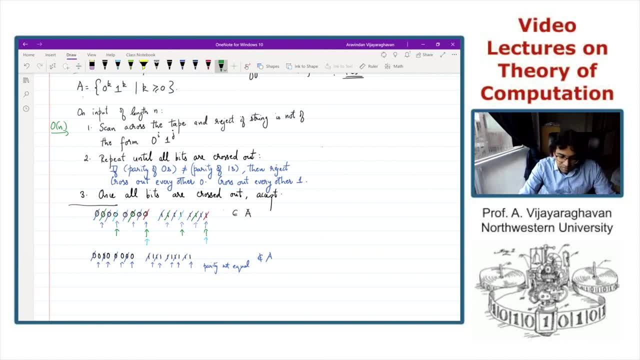 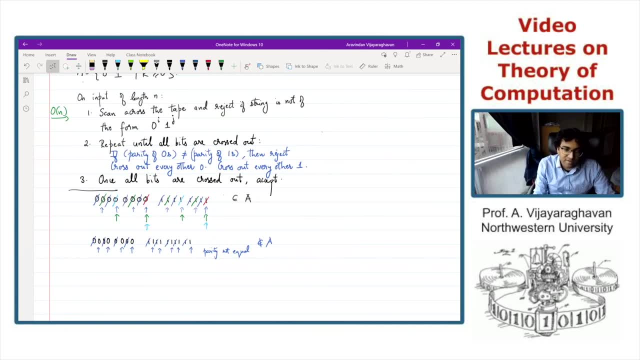 Okay, now let's look at the second step. Okay now, the key thing here is that in every step, okay, in every iteration- I mean this whole sequence of crossing out things, I mean this whole sequence of crossing out things- half of the input is scratched out. 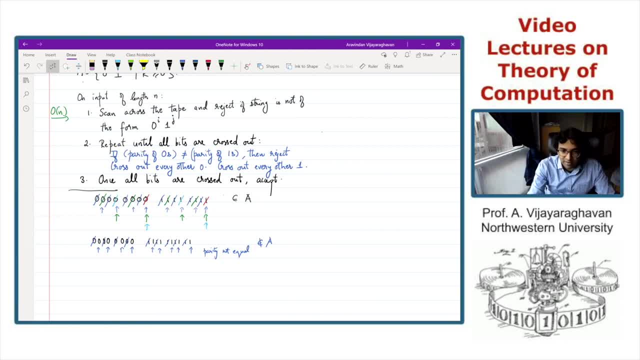 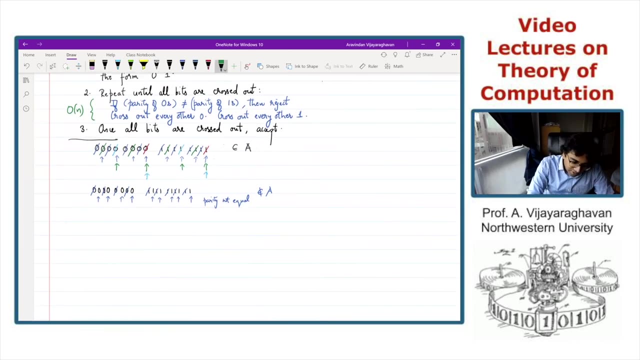 Okay, so in every iteration you may take order and time. okay to go across the input. It's essentially a scan, okay, But half of this is scratched out and half of what is remaining is scratched out. So the time complexity in total. 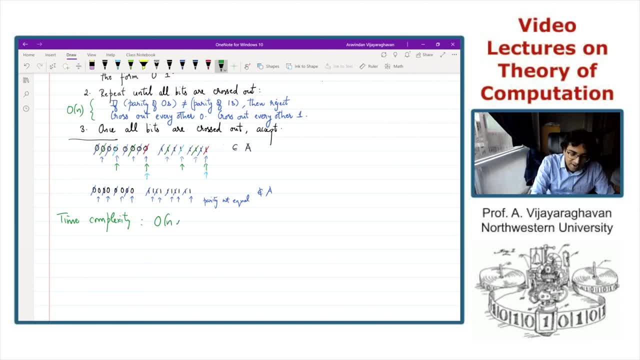 is, you may take order and log n. okay, Since in every iteration half the input is scratched out, At least half the input. it could be more okay. Hence there are only order log n iterations, And this gives a time, complexity bound of order n log n. 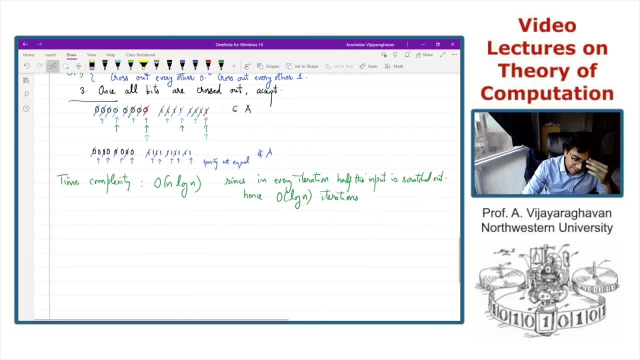 Okay good, So this says that A is actually in time of n log n as well. Okay good, It is in time n squared, but it is also in fact in time n log n. Now here are a few remarks about this. 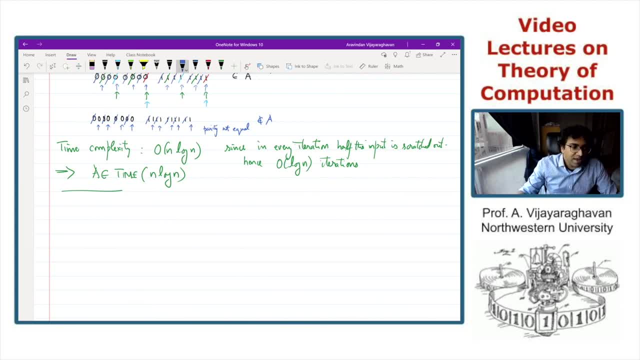 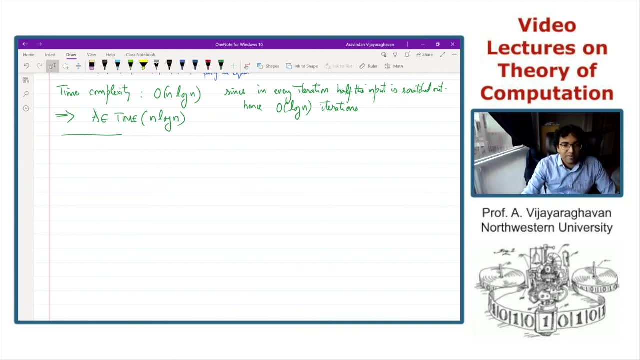 Okay, It turns. you could ask: well, could it actually be? could there be an even more efficient algorithm? Okay, maybe it's in time complexity class. you know time of n. Maybe there's an order n time algorithm. okay, 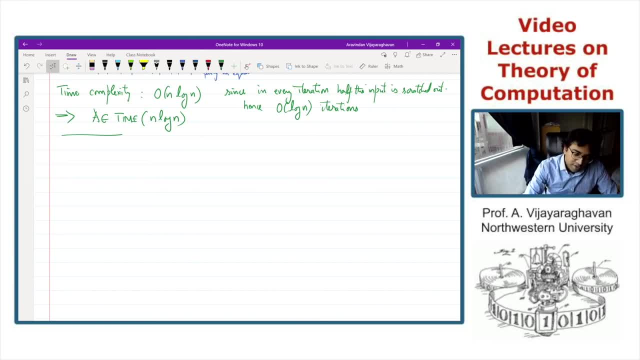 Or maybe something between n and n log n or even smaller. It turns out that the time complexity is actually n log n And in fact you can show that you know any one tape during machine, which is the usual Turing machine that we have looked at so far. 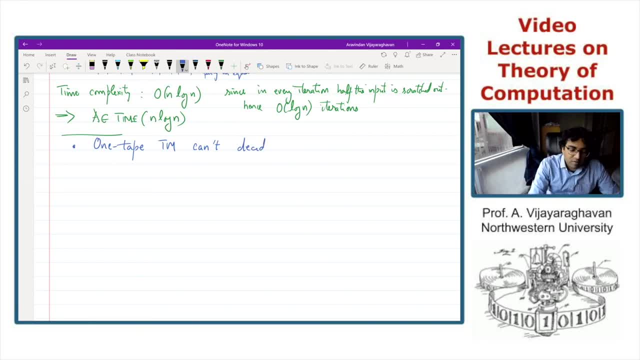 can't decide A and little o in any smaller time. that is asymptotically smaller time In little o of n log n. it's impossible. Okay, this is something that can be shown and we're not gonna show it here, okay. 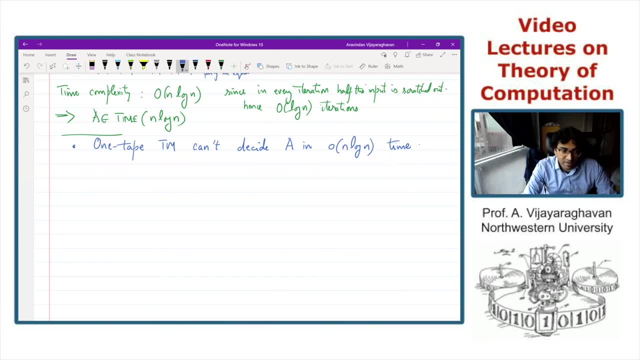 And in fact there's something stronger that you can show, and this is an exercise in SipSip's book, because you know, since it turns out that the only languages that can be for which you can construct a one tape Turing machine, 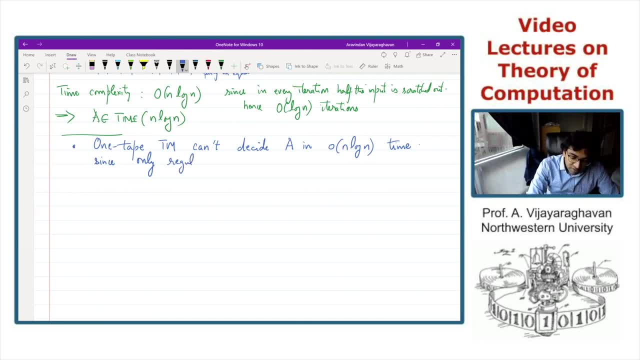 that decides it are regular languages. okay, So sorry, one tape Turing machine that decides it in little o of n log n time. Okay, regular languages. Okay, regular languages. Remember n log n. Yes, n is the size of the input. 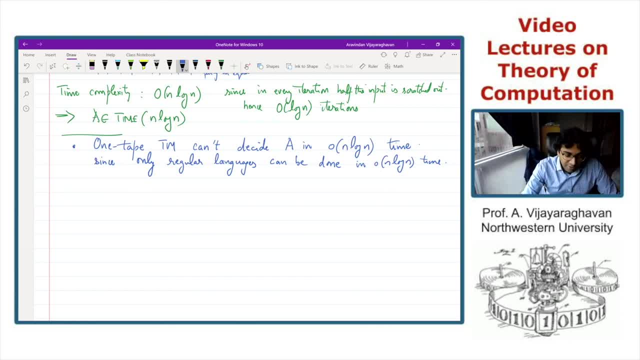 So this is an interesting lower bound for one-tip Turing machines. And here's another point which is something that you may have seen in one of the lectures already in Turing machines. But recall that regular languages are precisely those languages where the number of states is finite. 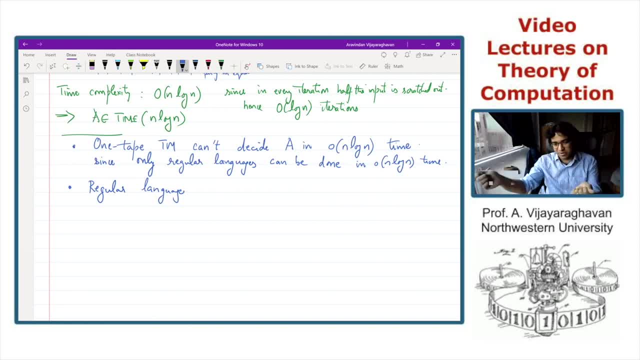 It's really a constant And you just have your input and it goes through the whole input like a stream. So regular languages are exactly those languages for which you can construct Turing machines which only need order and time. So what I'm really saying is that regular languages are 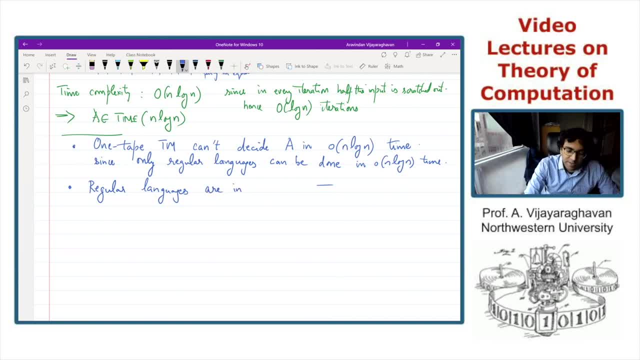 in time And the complexity class time of n. So what this is really saying is that between time n and time n log n, just less than n log n, a little of n log n. there's really not that much power that you get. 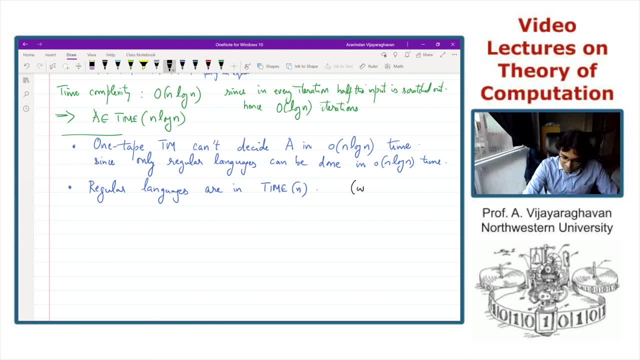 So, by the way, I'll leave this as an exercise to figure out formally why this is the case. But once you go to n log n, you're going to get this, And then you are starting to recognize these languages like a bunch of 0's followed by an equal number of 1's. 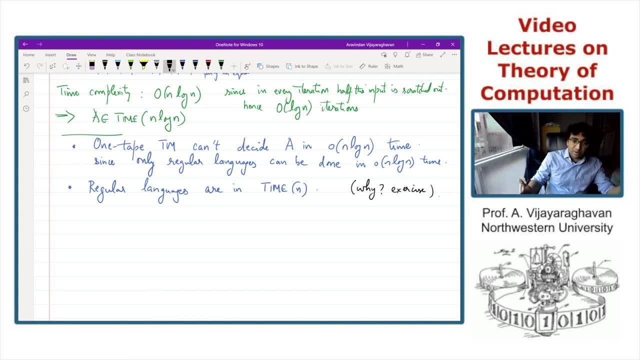 And so you seem to, which is certainly not regular. So you seem to get much more power. So good, So you see that there is more power that comes from going from order n to n log n. Do you always get more power now when you go from, let's say, 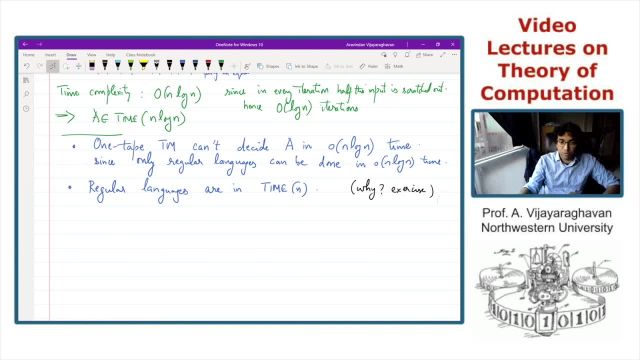 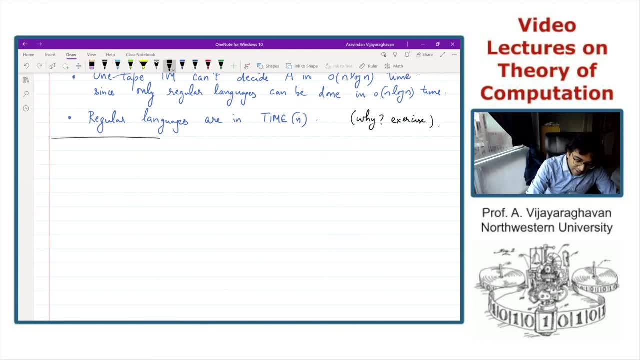 n log n to n squared, n squared to n cubed, and so on. OK, And this leads us to what is known as the time hierarchy theorem, which really tells you that with more power, with more time, you get more power. 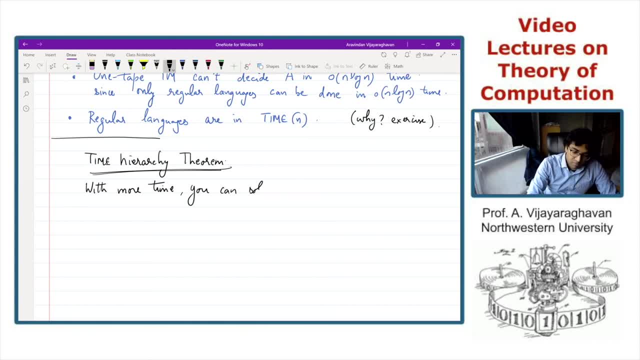 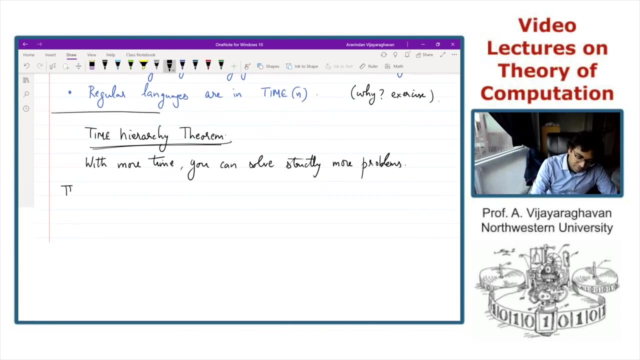 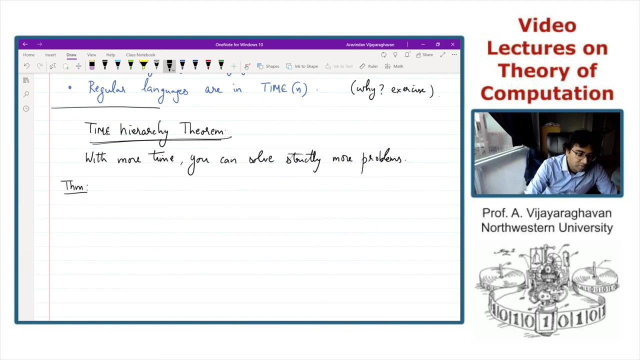 So you can solve strictly more problems. So here is the theorem And in fact we are not going to see a proof of this theorem. I'd encourage you to read SIP-SER to see a proof of this theorem. So basically, here's the theorem. 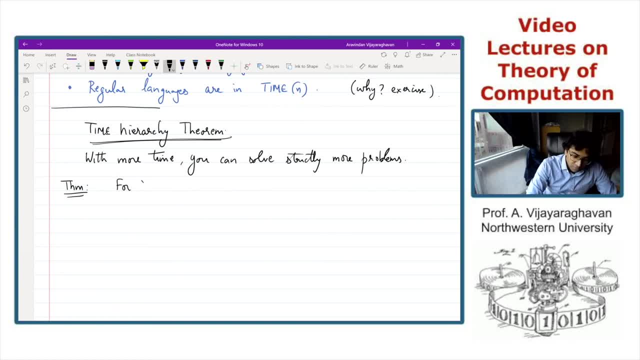 For any, for reasonable f and g, and there's a very simple condition that you need to satisfy: where g of n is some larger function than f, But in fact something slightly, I mean quite a bit. I mean just a little bit more larger than just saying: 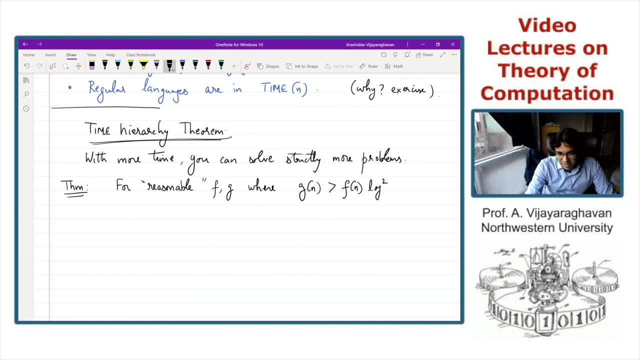 that g of n is greater than f of n. you want it to be larger by an extra amount, OK, Which corresponds to this log squared n. OK, Then you can say that the time complexity class that corresponds to f of n is a strict subset of the time. 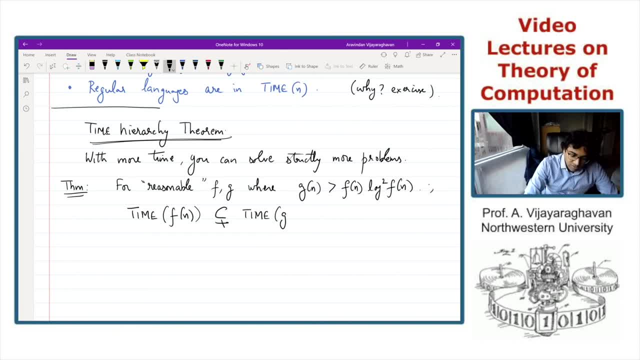 complexity class. that corresponds to g of n. OK, So g of n is something that is a little larger than f of n, OK. Now, the fact that it is a subset is not the interesting part. The interesting part is the fact that it is a subset. 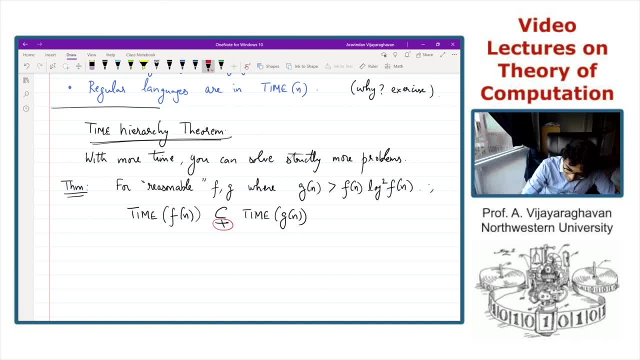 OK, So g of n is something that is a little larger than f of n. OK, But it's a fact that it's a strict subset. OK, So it says that it's not equal, And that's the interesting part, And this proof is using, in fact, the proof. 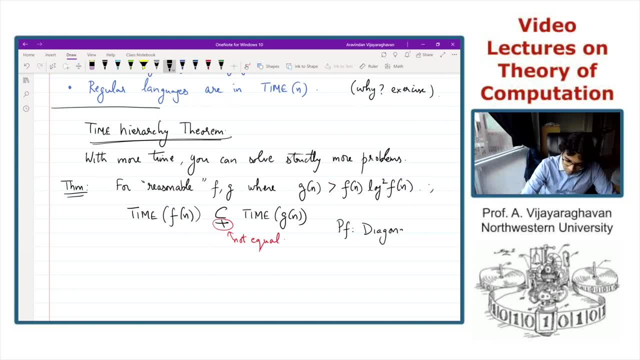 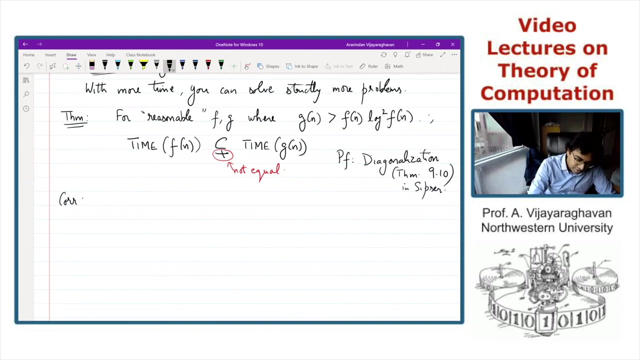 is using diagonalization, And this is actually theorem 9.10 in SIPCEL, So an increase. I encourage you to look at it if you are interested in the proof. Now here's a simple corollary of it, which I think is quite interesting and useful. 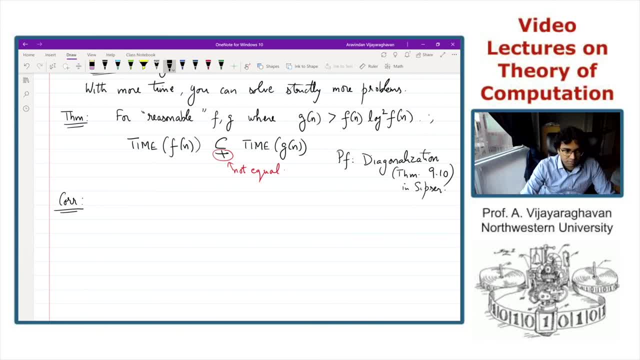 And I mean, yeah, this is a good way to remember it as well. So, corollary, you can think about these functions, f and g- as, for instance, you can think of f as being n and g as being n squared. 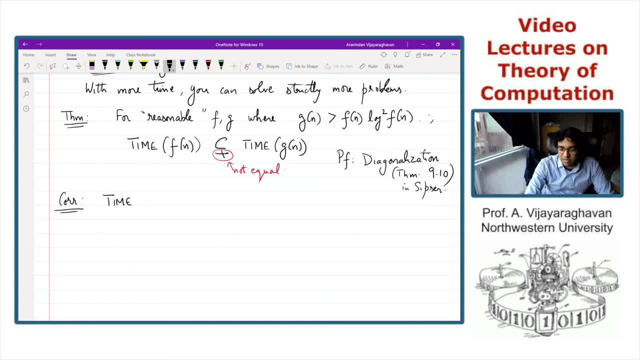 Now the condition is just saying that n squared should be much larger than you know f of n, Which is n times log squared n, which is true. OK, So this really says that time of n is a strict subset of time of n squared. 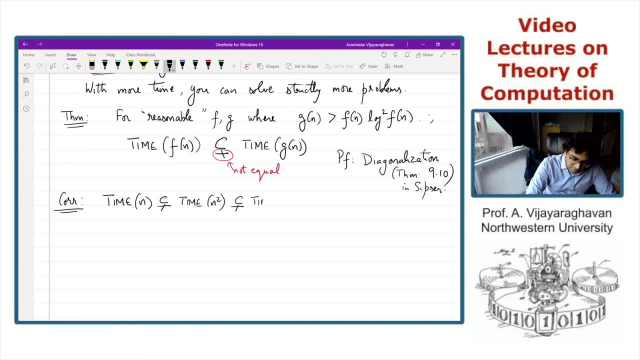 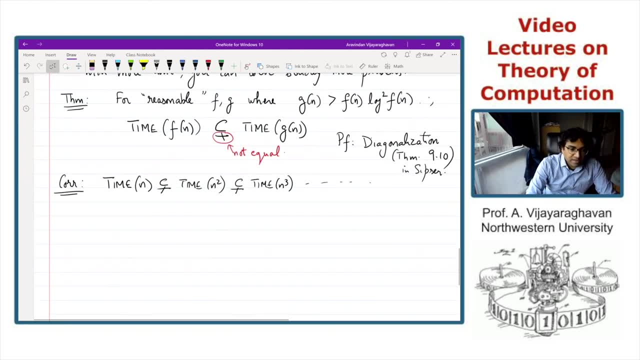 And similarly, the time of n squared is a strict subset of time of n cubed, and so on. OK, So this really says that there's an infinite hierarchy And if you look at this, you can see that there's an infinite. 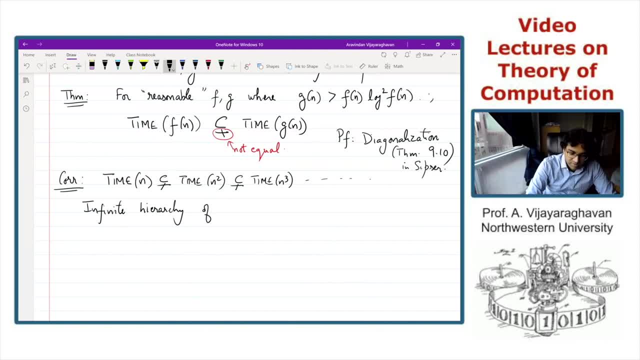 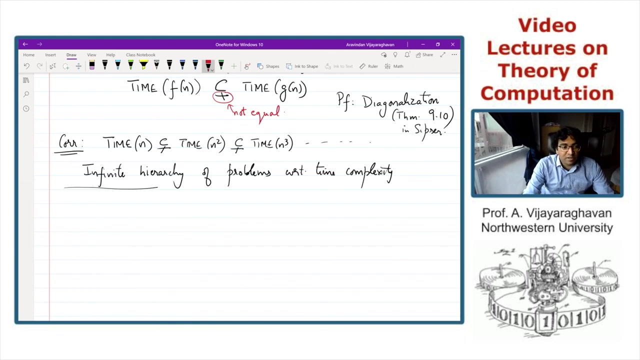 hierarchy of problems. OK, with respect to time complexity, However, I mean this only tells you that there are languages that belong to, let's say, time complexity class n squared. that don't belong, sorry, that belong to time complexity class. let's say: 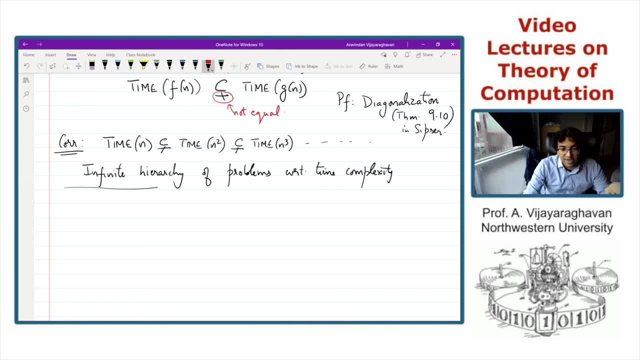 n to the 10, that don't belong to time complexity class, let's say n squared, or even n to the 9,. OK, But I mean. an interesting question, which is in fact quite open, is: are there natural? 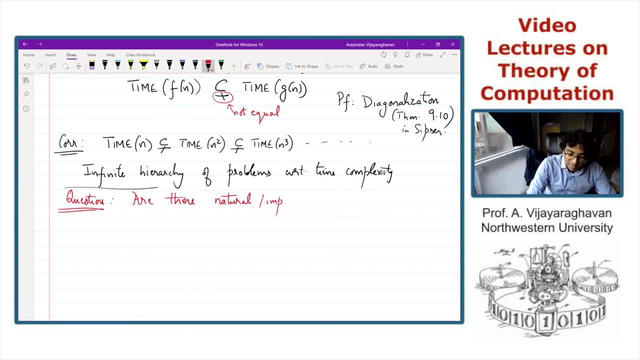 you know I mean important problems that we actually care about, That are high up in this time hierarchy. OK, so this time hierarchy theorem only tells you that there are languages, but I mean, these are probably not the languages that we think. 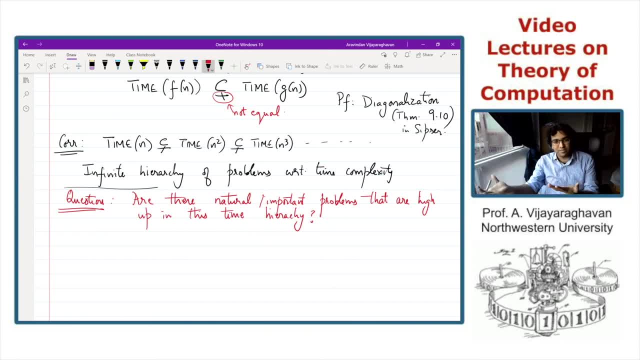 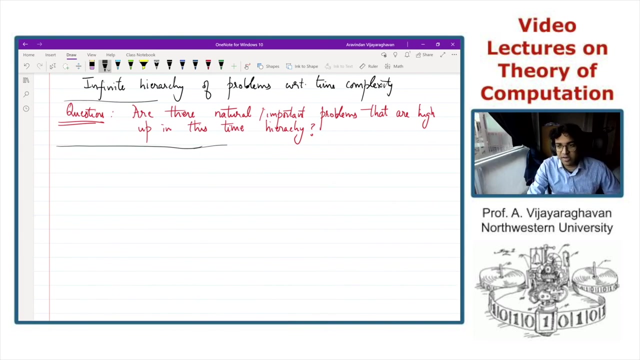 as you know. i mean, these are, these don't correspond to natural problems that we care about. okay, particularly higher up and higher, and figuring out these kind of problems is actually a- i mean, a research challenge. so now let's move on to this question of: okay, so we have defined time complexity with respect to 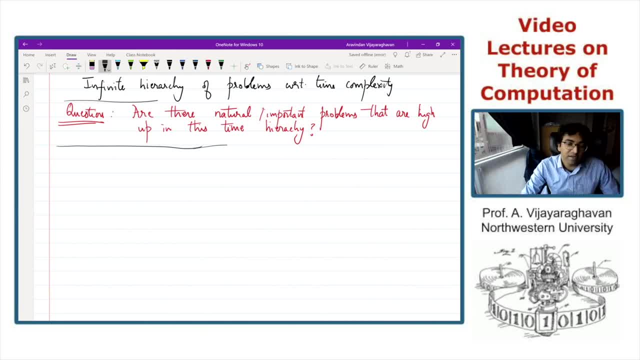 single tape curing machines. okay, we have seen that there are many other variants of curing machine, for instance multi-tape curing machines and so on. now, do these concepts, you know, like uh, extend? i mean, is there some robustness with respect to uh time, complexity, i mean, across these different models that we saw with respect to, let's say, computability? we saw 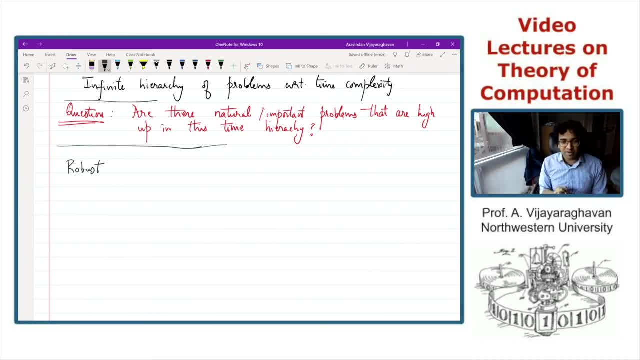 that you know the set of all languages that can be computed or decided by turing machines. i mean, it doesn't really matter whether you're talking about single tape or multiple tape, and that's. is that the same when it comes to a more fine-grained way of measuring, uh, time complexity, so robustness across different? 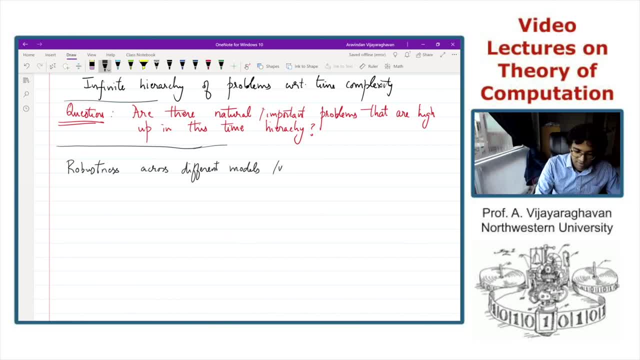 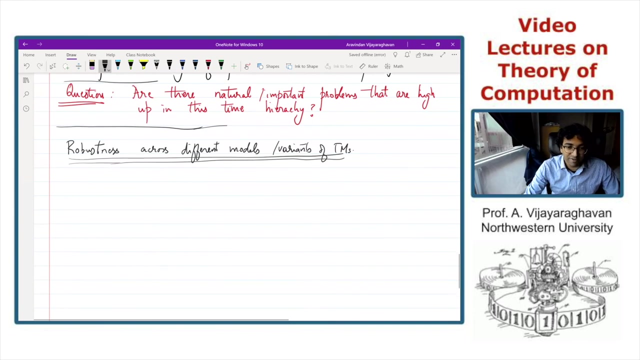 models or variants of turing machines. okay, so that's the next topic that we're going to explore. okay, to answer this, uh, very succinctly. well, it turns out that, the time from time, complexity can actually change when you look at a slightly different variant of turing machines. okay, so let's look at an example. 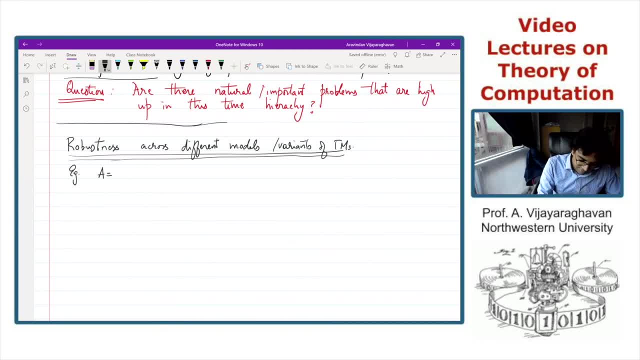 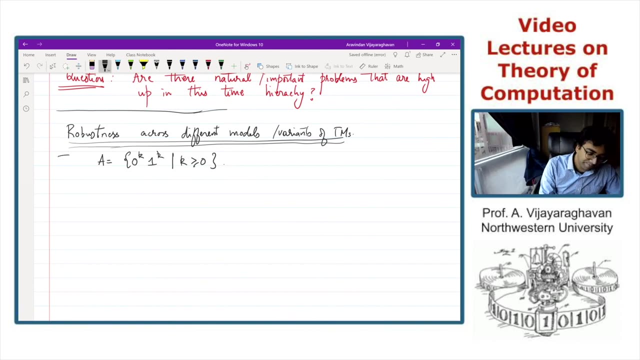 let's look at our favorite example, which is the language consisting of. you know this language a that we've looked at a couple of times before. okay, so here's a theorem um the language a that we've looked at a couple of times before. okay, so here's a theorem um the language a. 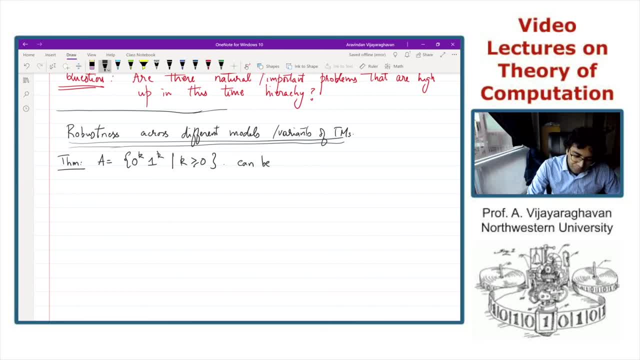 that we've looked at a couple of times before. okay, so here's a theorem: um, the language a can be decided in order and time using a two tape turing machine. okay, recall that with one tape it's impossible to do that. you can't even go below. 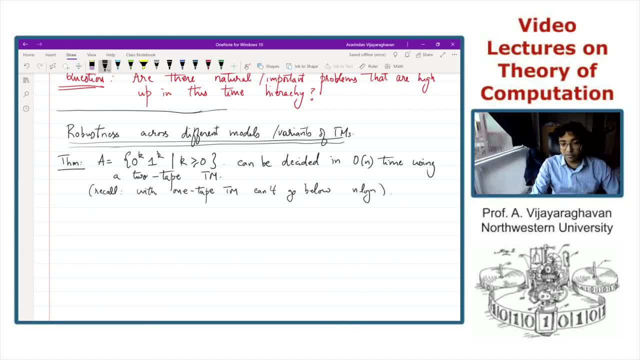 and log in. okay, but for the two tape cutting machine you can actually design a simple algorithm which just takes order and time. okay, and here is the okay. so here's the pseudocode or the proof idea. just here is the pseudocode. okay, and here is the proof idea. 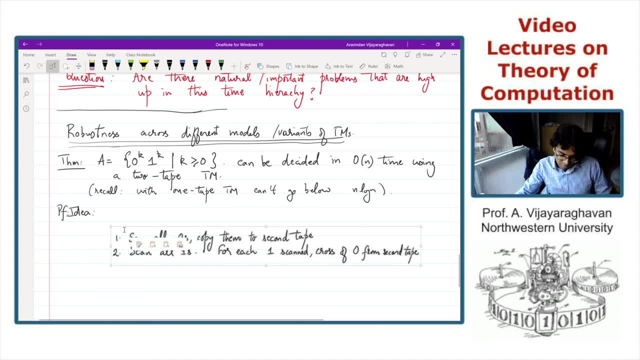 let me on this question. so let me actually just copy paste the sort of code to save some time. so, like before, on input of length n. so the first step is just gonna be tecnología: have two tapes, okay, now control. so we just scan all the zeros, okay, and then copy them onto you. 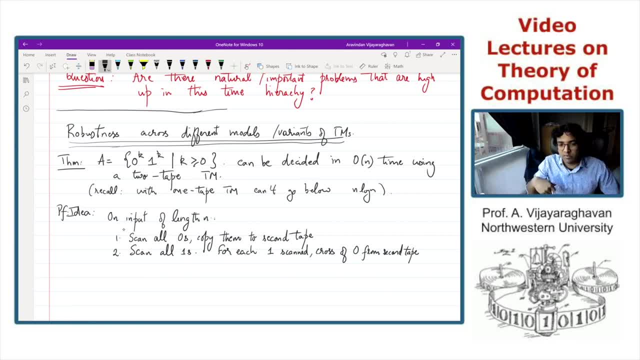 know the second tape. okay, so just uh go through all the zeros that come at the beginning. okay, so again, we're only going to look at all the zeros that come before the first one. okay, just uh scan through them and then copy all of them onto the second tape. 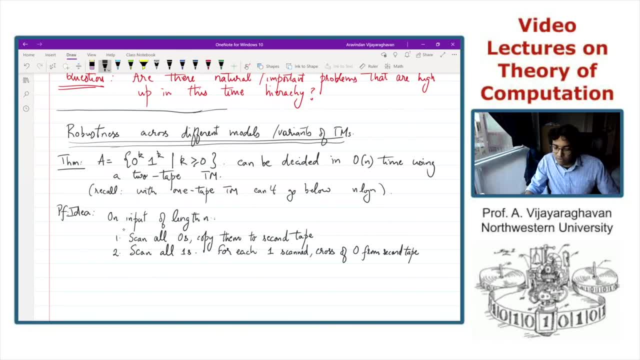 okay, okay, now what you do is for? uh yeah, if you want, you can just add another step, which is, you know, just ensure that it is always in the form but the zeros, followed by a bunch of ones, so you can just scan all the zeros, put it into the second tape, and this only takes order and time. 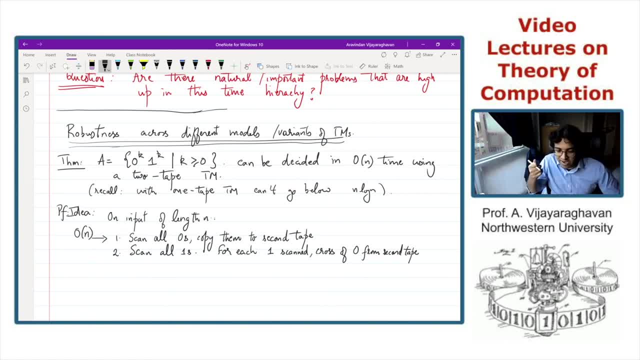 and now what you do is you now scan all through all the ones and for each one that is scanned, cross off a zero from the second tape. so remember that you have two heads because you have two tapes. right, and now you know you. when you cross over zero, you again, you also cross over. 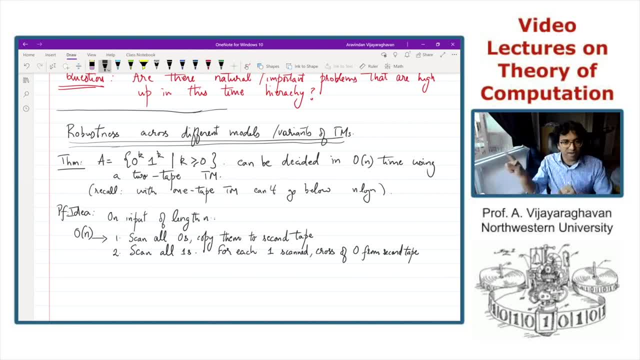 one and you move both heads right. so again, cross over zero, cross over one, and so on. so these heads go simultaneously and it's only going to take order and time, okay, so the time complexity, so time taken- is order n and the time complexity is order n. 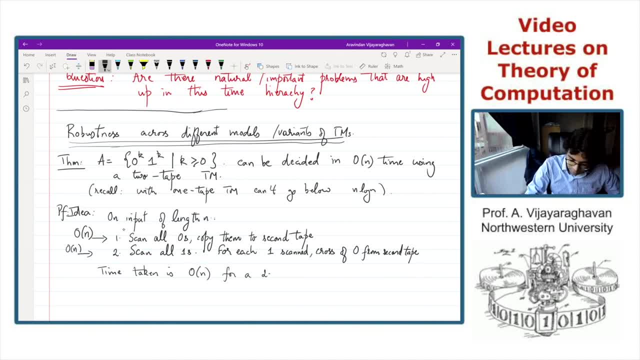 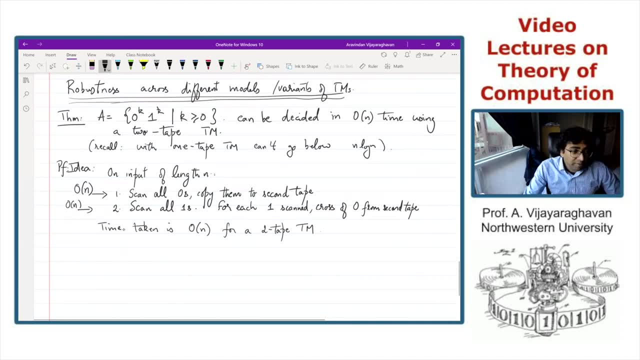 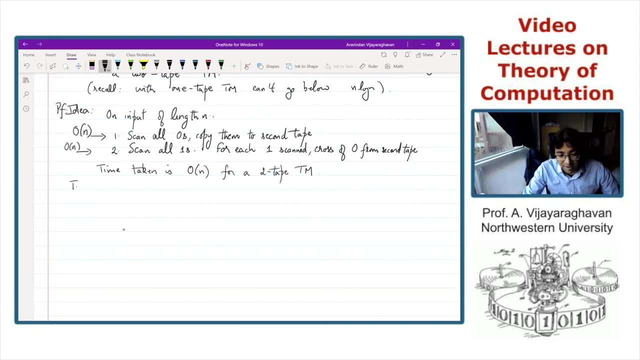 for a two-tip turing machine. okay. so the takeaway is that, uh, you know this, uh, so, in fact, this gap can be um in um uh can be larger too. okay. so the takeaway is that, time complexity associated with you, you will get uh um. okay, so, in fact, this ability is the same regardless of 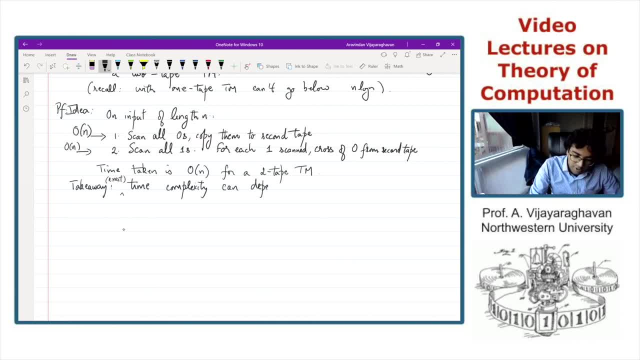 the time complexity. so let me say that the exact time complexity may depend can depend on the model. okay, and in fact this gap can be quadratic. potentially gap is, for instance, the language corresponding to, you know, repeated strings of the form w followed by w. okay, this is again not a regular language and in fact, for this as well, you will, you can. 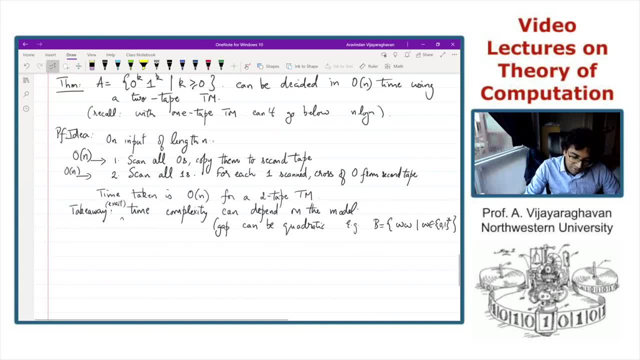 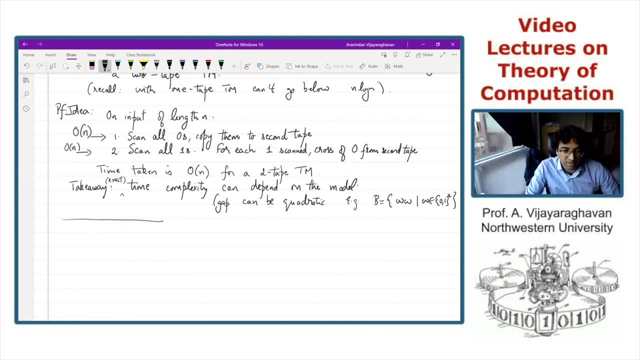 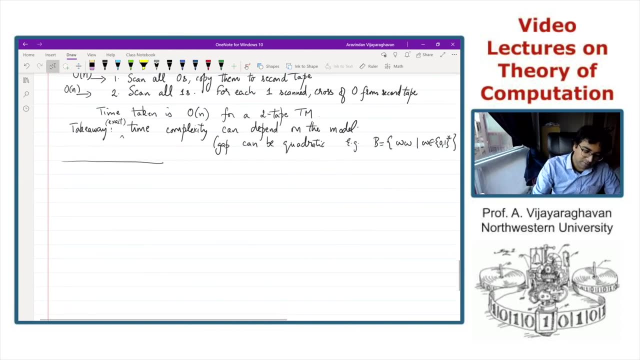 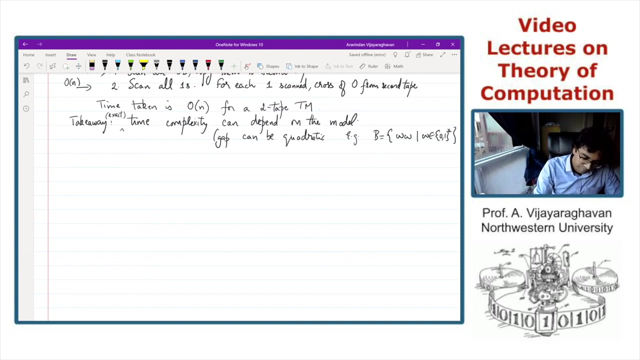 show that the gap is quadratic, but what we're going to see now is that, while this gap can be quadratic, it can't actually be worse than that. so that is really- i mean, it's not quite the time. complexity is not exactly the same, but there is an approximate equivalence, okay, okay, let me just: yes, 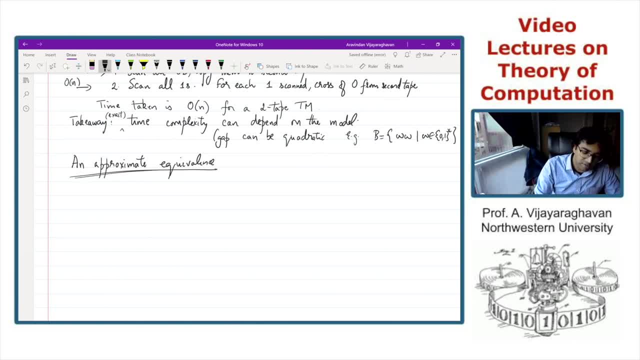 so an approximate equivalence exists. okay, and this is a theorem, and this is not just for two tape turing machines, for multi-tap turing machines. so it's true, for multi-tap turing machines, let t of n be a function of n. okay, and you know, we are going to assume that you know it's, it's at least n. 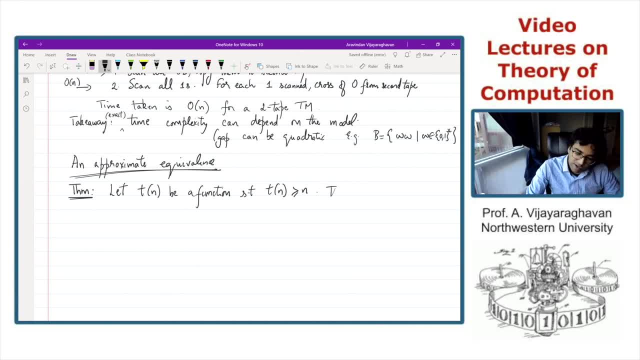 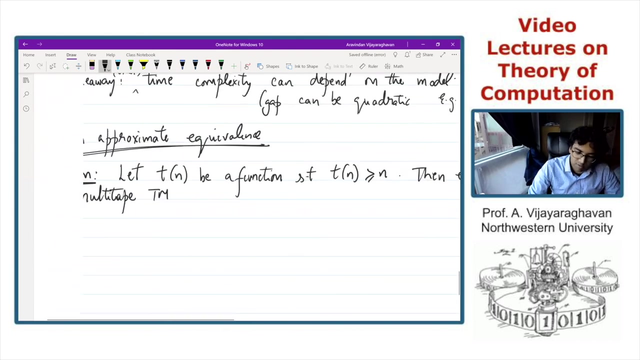 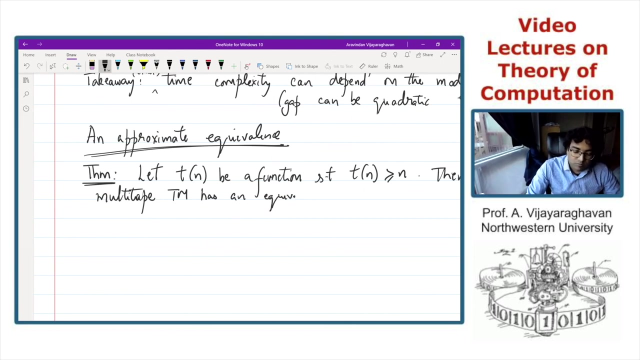 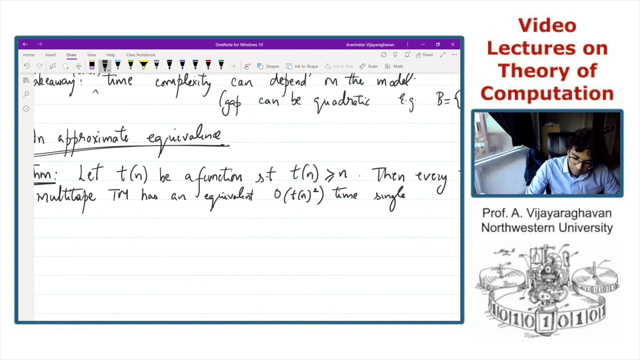 okay, this is a very minor condition, then every t of n time multi-tap turing machine has an equivalent of t of n to the whole square time, and let's assume you know this is a whole squared time: t of t of t of the whole squared. 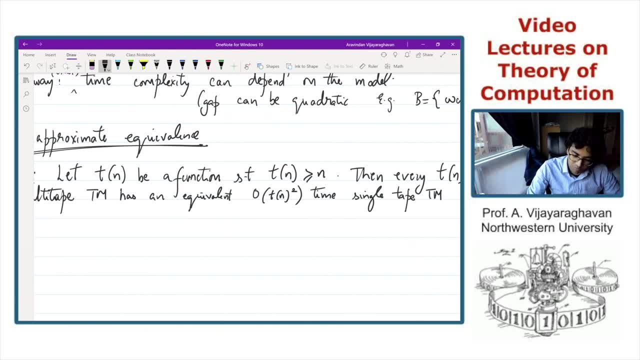 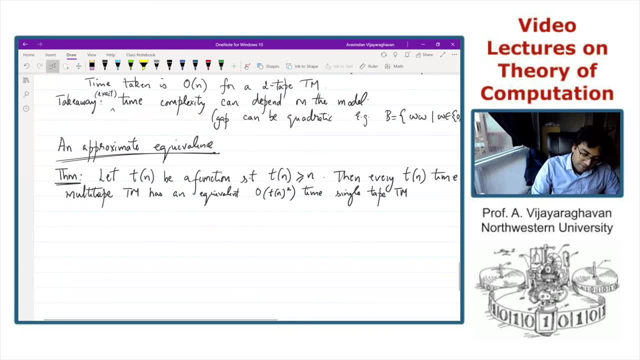 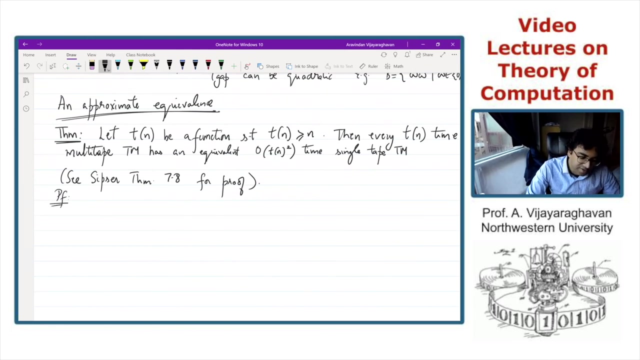 order t of n, the whole squared time. single tape turing machine. Let's see SIPSR, theorem 7.8, for proof. Okay, And really I mean, the proof is not very complicated, It actually just uses the same simulation that we saw, for you know, 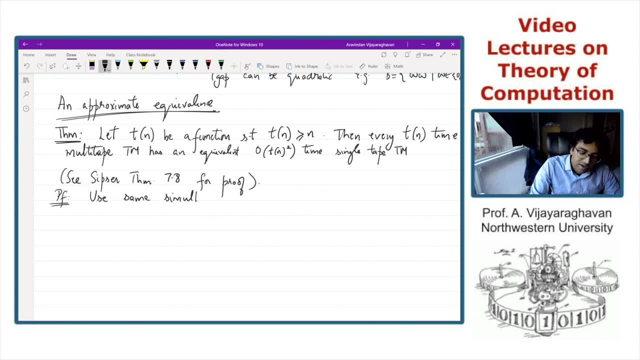 we had a simulation argument that showed that multi-tape Turing machines and single-tape Turing machines compute the same, I mean can recognize or decide the same languages. Okay, And you're just going to use the same proof? Okay, So we're going to use the same simulation. 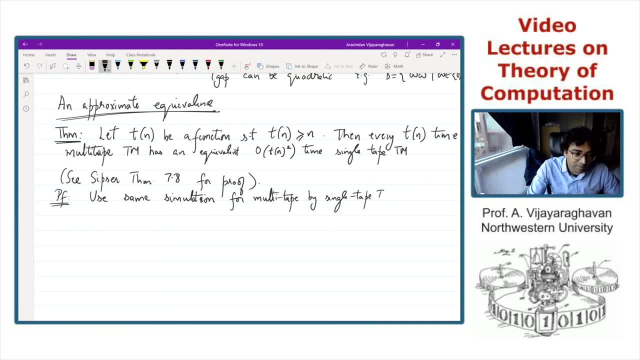 argument that we saw for simulating a multi-tape Turing machine by a single-tape Turing machine And you can actually show that each step in the simulation Okay. So for each step of the multi-tape Turing machine, okay, that simulation will require at most, you know. 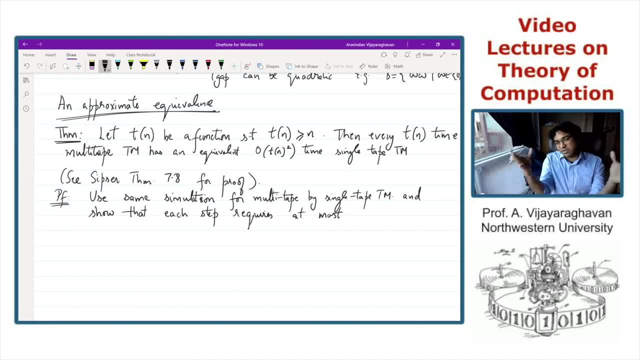 the amount of time. So the amount of time that corresponds to the total length of all the tapes, the sum of the lengths of all the tapes And the sum of the lengths of all the tapes is also, at most, T of n. So for each step of the 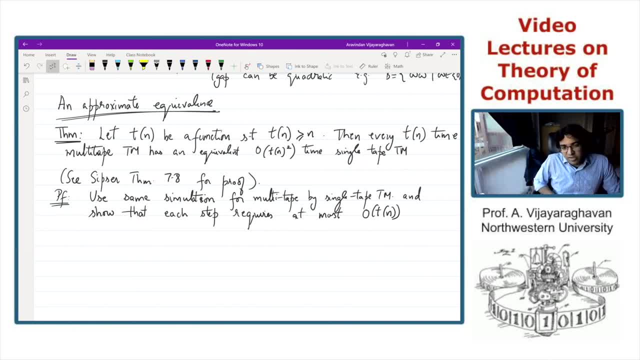 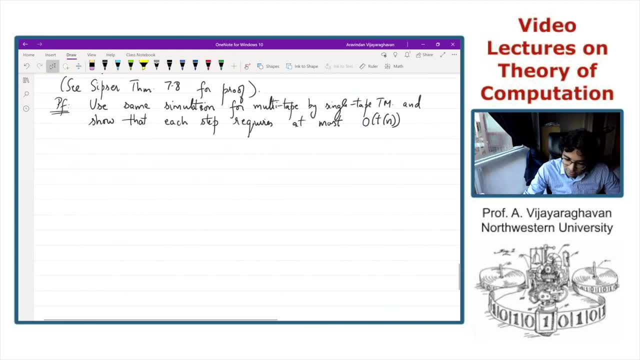 for simulating each step of the multi-tape Turing machine. you can do this in time, which is at most order T of n Okay And there are T of n steps, So this in total gives you order T of n squared. 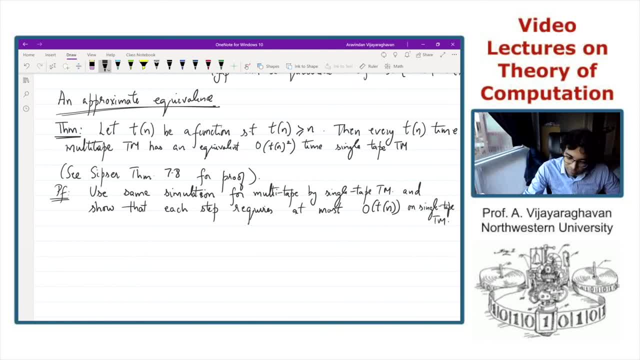 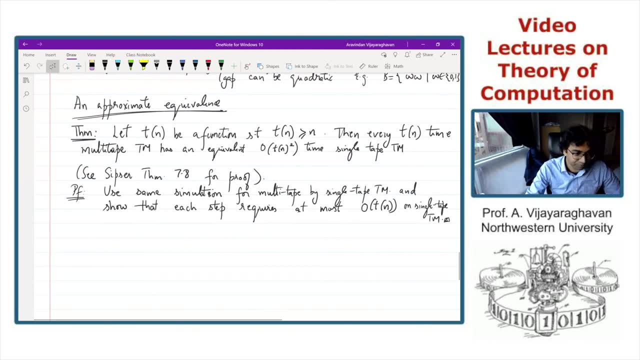 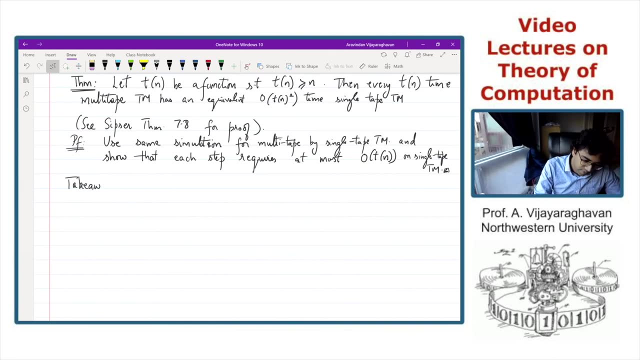 But I'm not going to go into this full proof because it goes. looks into the simulation argument again, Okay, Which we have seen already. Okay, Good. So the main takeaway of this is that there is a robustness in the definition. 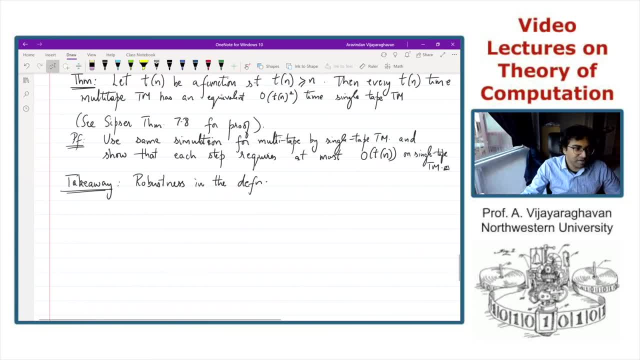 Okay, Okay. So I mean as a corollary, for instance: okay, you could say that. okay, suppose L is a language that takes, okay, you know, for which you can design a multi-tape Turing machine. takes time given by. 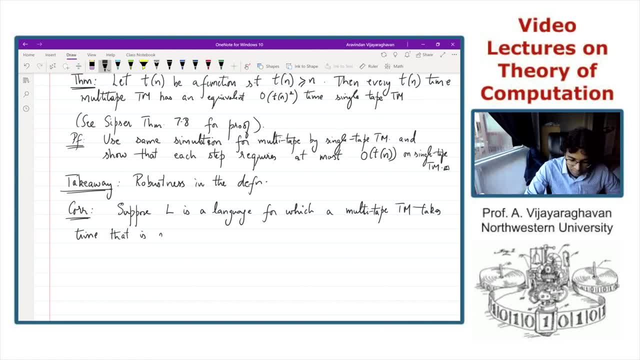 that is at most P of n, where P of n is a, a polynomial. Okay So this is a polynomial P of n. Okay, So then it also has. then L also has a single tape Turing machine. Okay So this is a polynomial P of n that has time complexity polynomial in it. 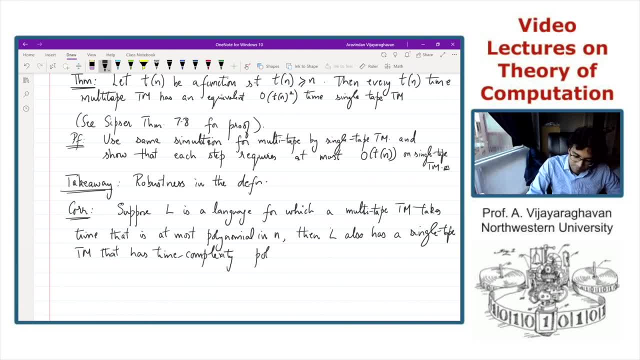 Okay. The reason is that there's only a quadratic blow-up in the time. complexity Okay Between a multi-tape Turing machine and a single tape Turing machine. So if you manage to show that there's a multi-tape Turing machine, which whose complexity is time, complexity is polynomial. 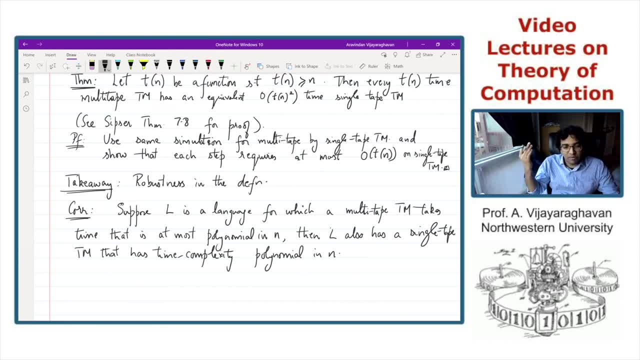 then that also means that there's a single tape Turing machine, whose time complexity is going to be that polynomial, the whole squared, which is also a polynomial. So there is this robustness in the definition. Okay, There's only a quadratic or a polynomial blow-up. 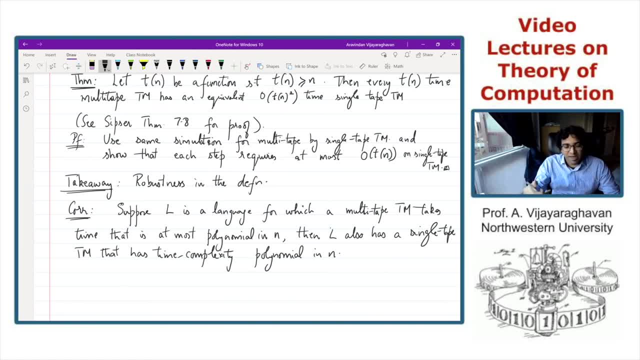 So it's really closed in this. Yeah, I mean, you could say that it's a polynomial, but it's not a polynomial. So it's a polynomial. So it's a polynomial, Okay, So, so, so, so. 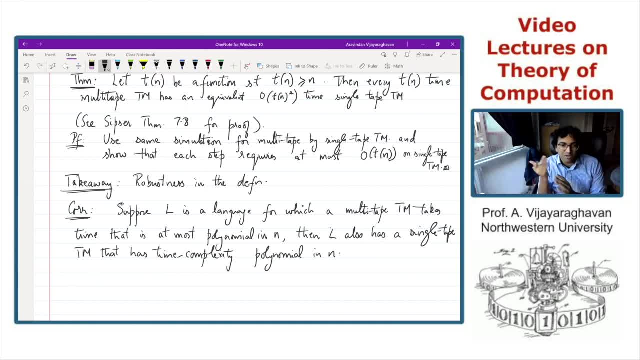 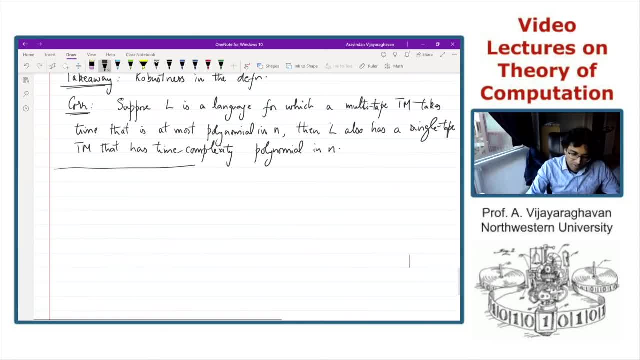 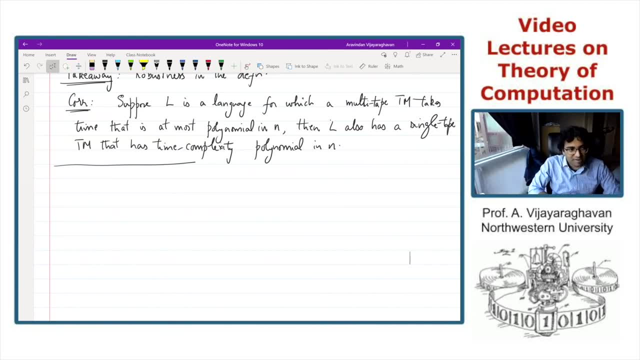 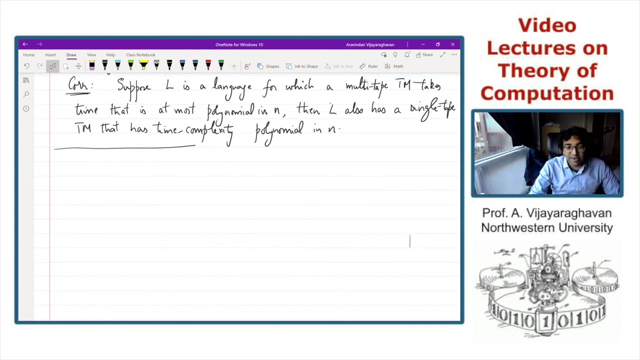 And this naturally leads to: so yeah, so there's this robustness across different models, and that's also true for other models of – various other models of Turing machines that you've seen, Okay, Except non-determinism, which we'll see, maybe in the next lecture. 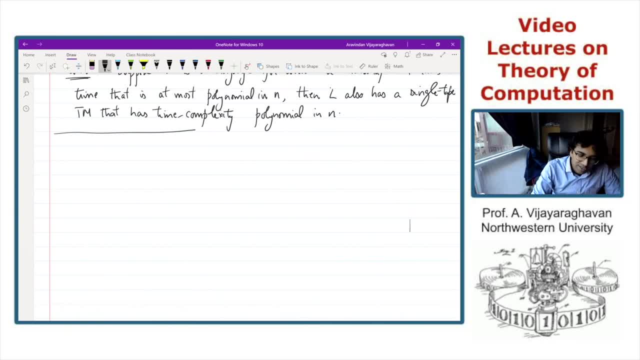 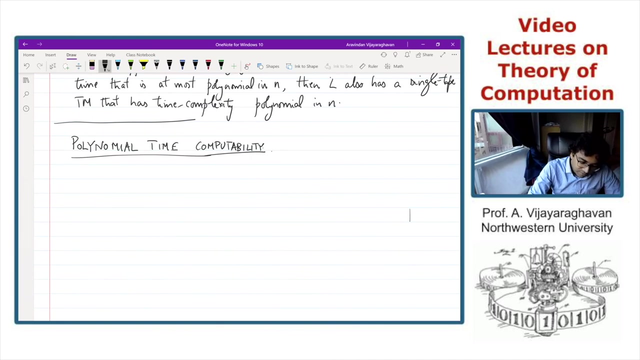 okay, so this, really this robustness in the definition leads to this class, which is, which corresponds to those languages which can be computed in polynomial time. okay, so. so this is the class which is which is called p. okay, it's the set of all languages that can be computed in polynomial time, so it's a union of all the languages that belong to. 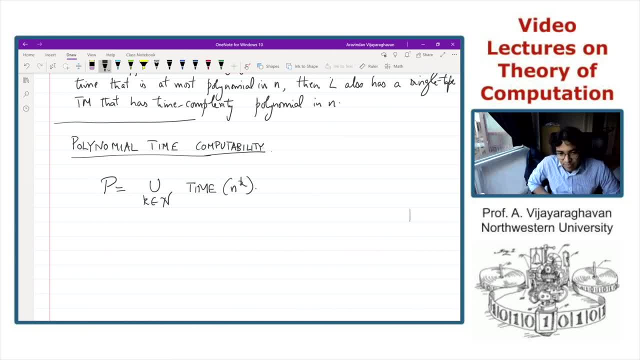 the polynomial time. so it's a union of all the languages that belong to the polynomial time. time complexity: class n to the k, for all natural numbers, k. okay, so you look at all the languages that belong to n, squared and cube, and i mean remember that this is an inclusion, right? so i 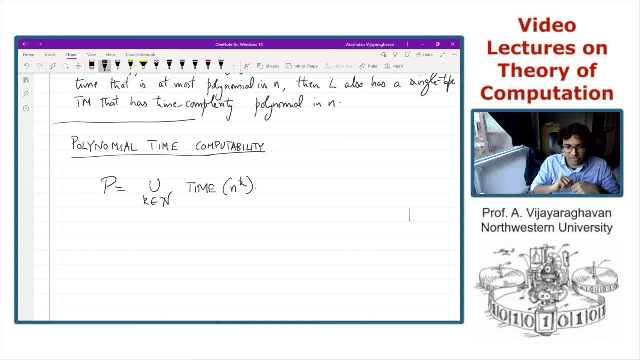 can i mean time? time of n squared belongs to time of n cube, and so on. you just want it to be, you know some? i mean you just want it to be inside the class time of some polynomial of n. okay, so the exponent this needs to be some constant. 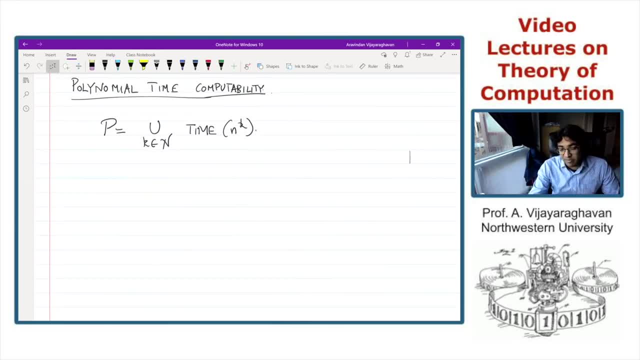 Good, And so as long as your language has some Turing machine that runs in polynomial time, it belongs to this class B, So this really captures a notion of efficiency. OK, So these correspond to all problems for which you can actually design an efficient algorithm. 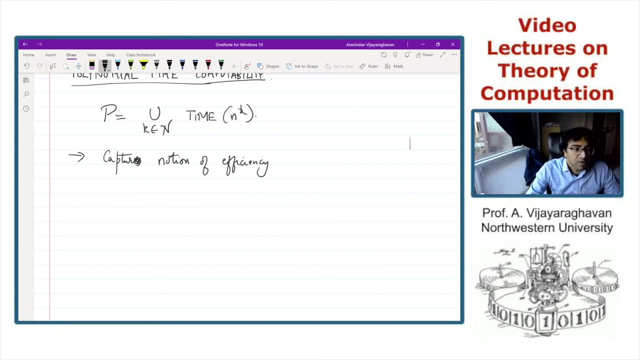 And the nice thing is that, because you only care about whether it is polynomial time or not, it is also robust across different models and definitions. So in practice we may care about whether it actually takes linear time or quadratic time and so on. That may be a big difference. 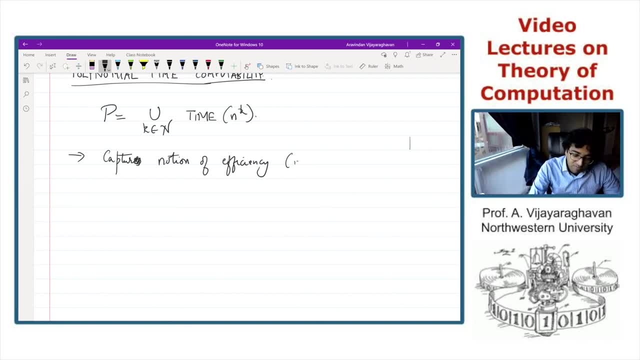 But up to a first-order approximation, this actually really gives you a very, very nice definition of what is efficient and what is not. So let me say that up to a first-order approximation, this actually captures all those problems for which you can actually design an efficient algorithm. 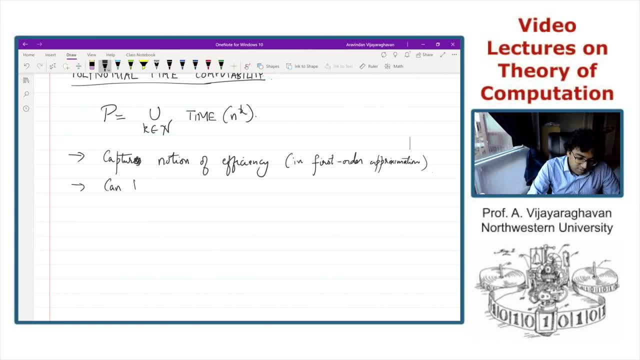 The nice thing is that it can also be defined in terms of other kinds of multi-taped Turing machines, for instance, or single-taped Turing machines, And they are really going to be the same thing, because we know that going from one to the other. 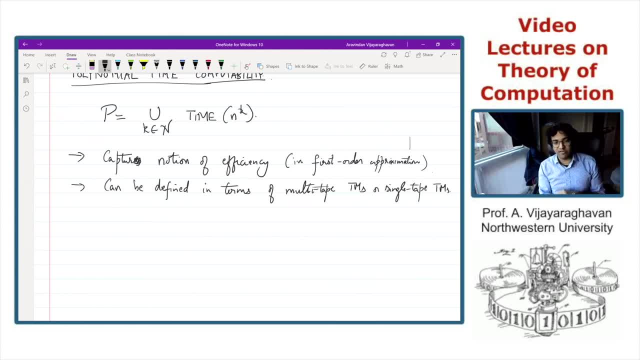 only involves a polynomial blow-up, which is fine according to this definition. So you could have defined it either in terms of single-taped Turing machines or multi-taped Turing machines. The definition is going to be the same And this notion is going to be an extremely useful notion. 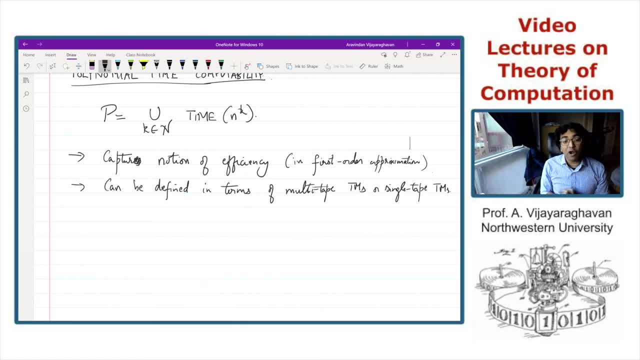 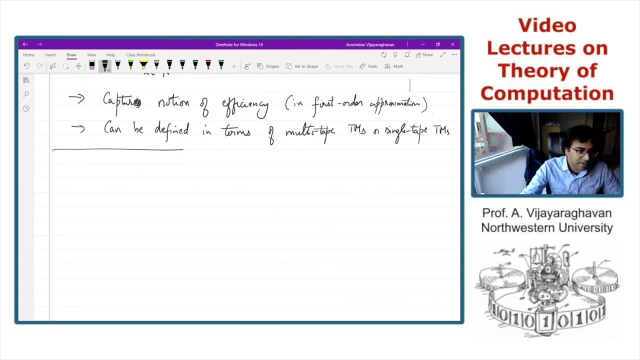 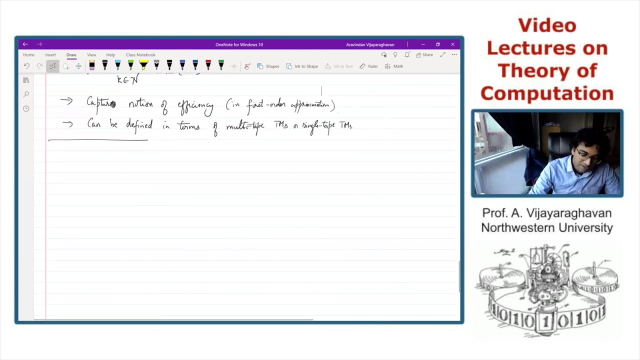 of efficiency And this has actually led to a lot of developments in this field of complexity theory And, in fact, the fact that there is this robustness in this definition across different models of Turing machine. it leads to something called the extended Church-Turing. 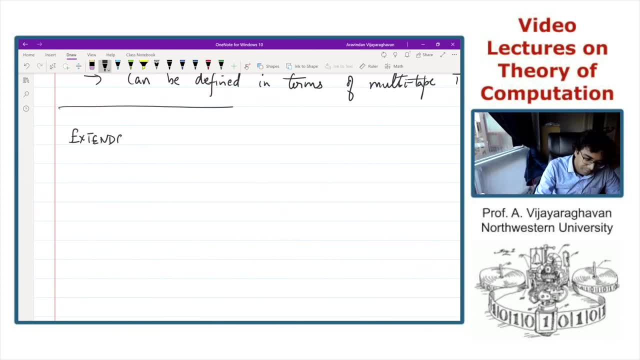 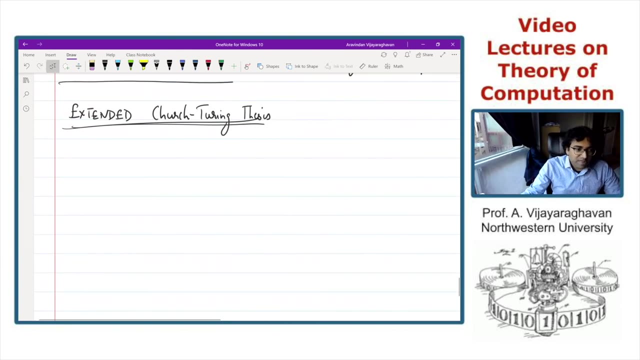 hypothesis, Or extended Church-Turing thesis, which says that this notion of efficiency, I mean it doesn't actually depend, I mean it actually captures your intuitive notion of efficiency in any model. So it really says that The Turing machine I mean more generally 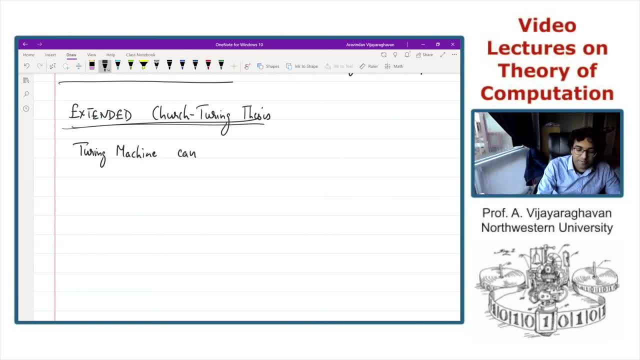 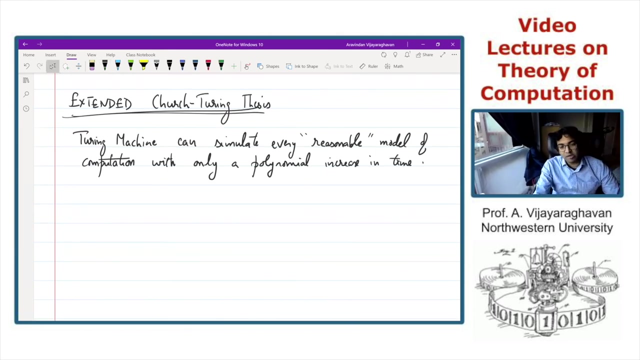 it says that a Turing machine can simulate every reasonable model of computation with only a polynomial blow-up. So it's a polynomial increase in time. OK, So this we have seen in the case of multi-taped Turing machines And it's true for some other variants that we have seen. 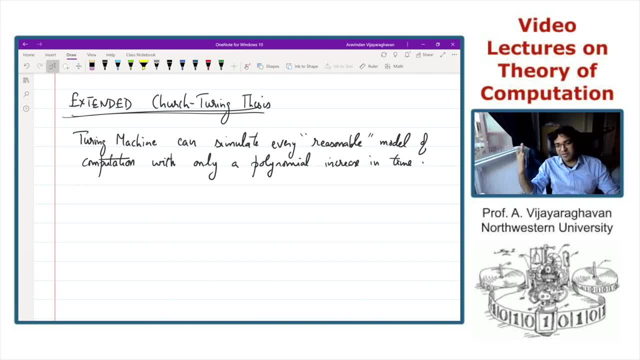 But the thesis really tells you that. I mean it's a strengthening of the original Church-Turing thesis, which was just saying that Turing machines can capture any model of computation that you can think about. Here it kind of quantifies it by saying that you can think: 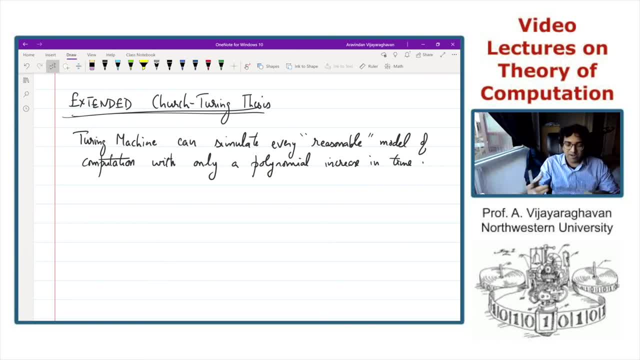 about any reasonable model of computation and Turing machine can simulate it with only a polynomial increase. It actually quantifies the amount of increase in the time. So this really tells you that I mean every intuitive notion of. So this really tells you that I mean every intuitive notion of. 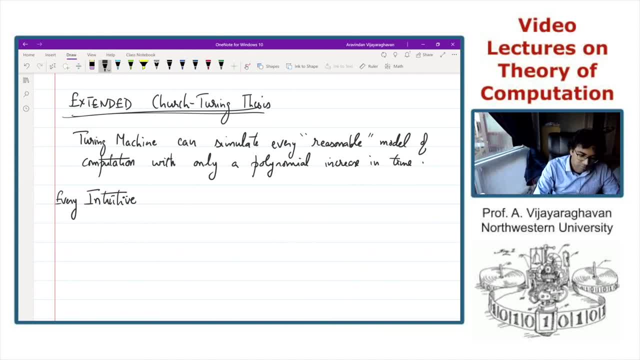 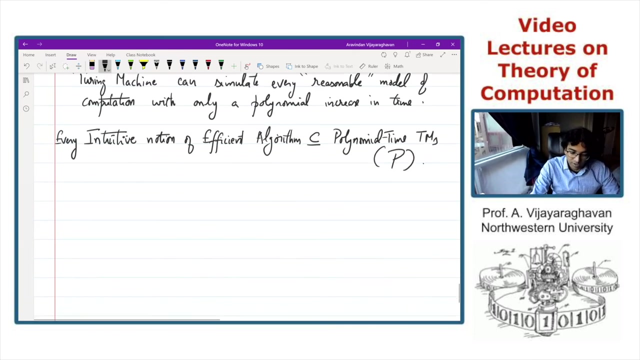 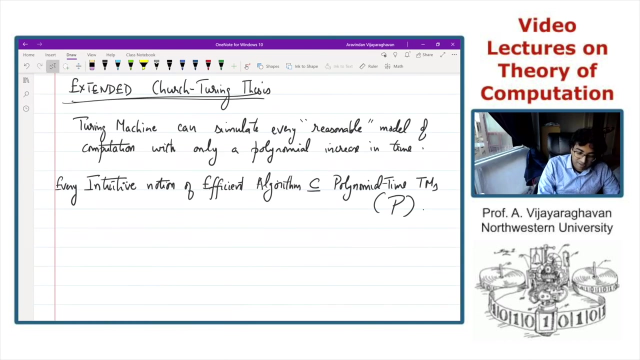 So this really tells you that? I mean, every intuitive notion of efficient algorithms is captured by polynomial time Turing machines, which is really our class B. I must say that this extended Church-Turing thesis is, I mean, it's a strengthening. 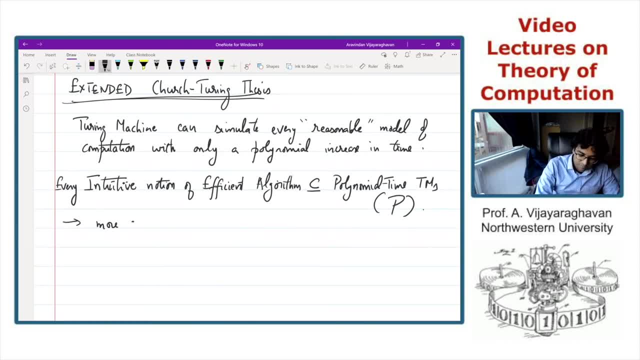 and it's also a little more controversial than the original Church-Turing thesis, And maybe it's particularly in the light of possible counterexamples, And one such something that's not still understood is quantum algorithms, Where we do know efficient quantum algorithms for problems like factoring, whereas we still 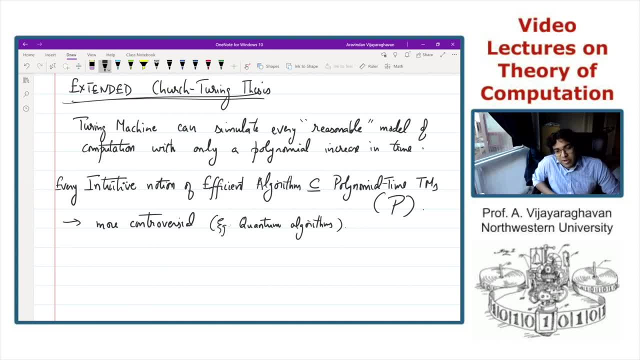 don't know any efficient polynomial time algorithm for factoring in the Turing machine model, the classic model of computation. And we don't know, A few years down the line someone may actually come up with a classical algorithm for factoring which will show that it's in P. But currently we don't. we don't. 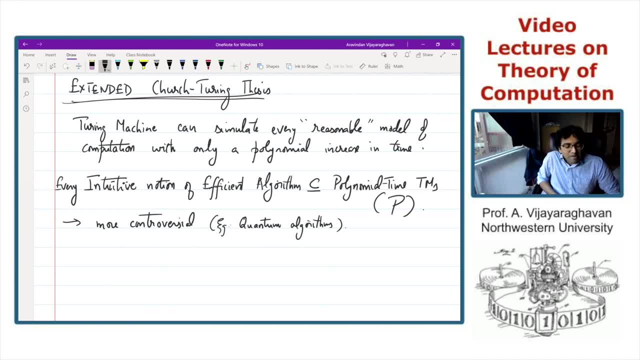 we don't know such algorithm, And we- I mean maybe people also believe that no such classical algorithm exists, In which case, yeah, this question is the validity of the thesis. But I mean, but there has been no contradiction to the thesis so far. 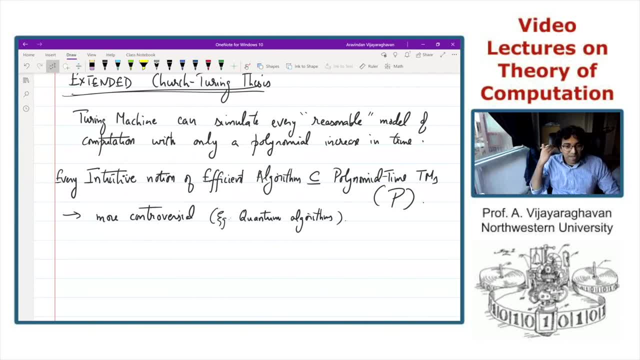 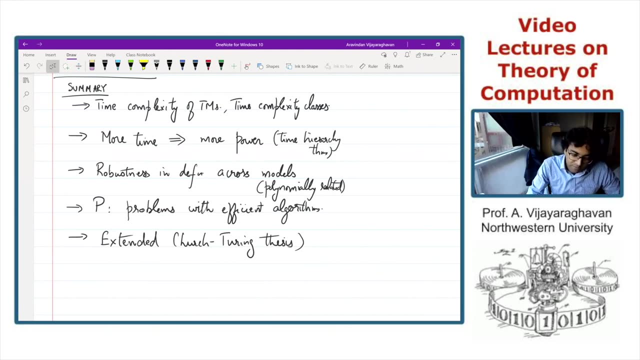 And this is the extended Church-Turing thesis, And this is, I mean, by and large. this has really stood the test of time as well. OK, so let's summarize what seen this notion of time complexity of Turing machines, And we also define time complexity classes. 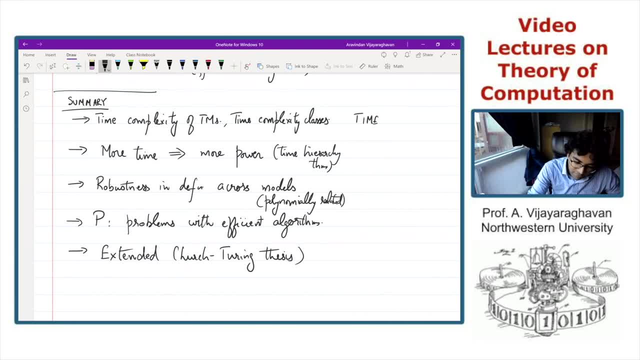 These were the classes of the form time, of some f of n, And we saw that more time corresponds to more power, And this is something that we saw in the context of the time hierarchy And this is something that we've also used in some of the other classes as well. 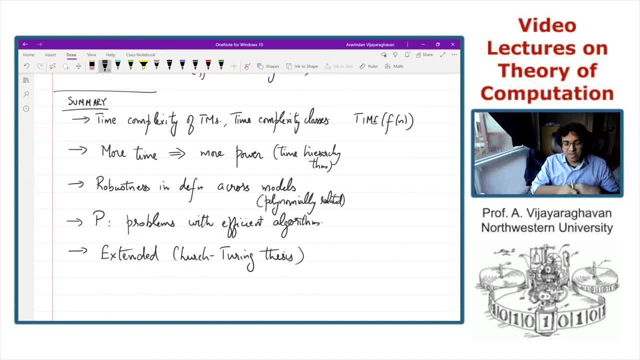 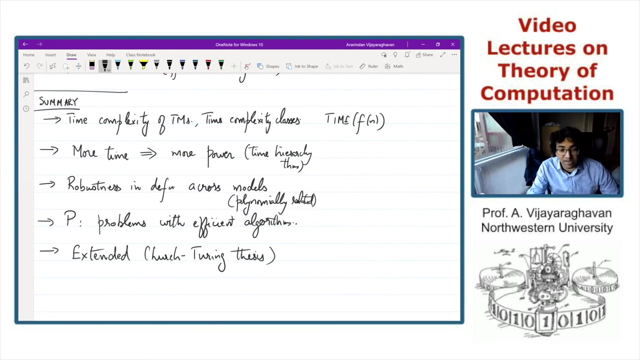 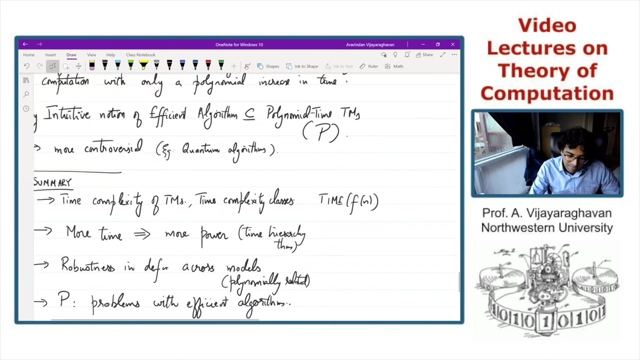 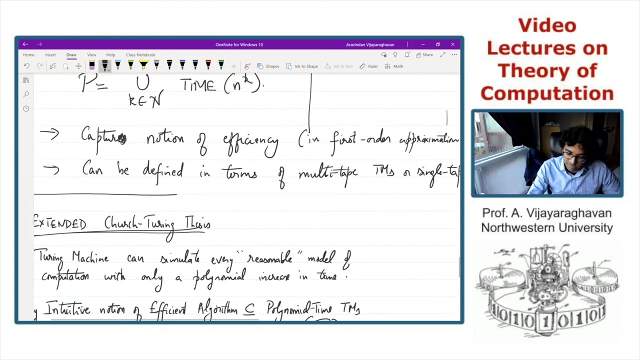 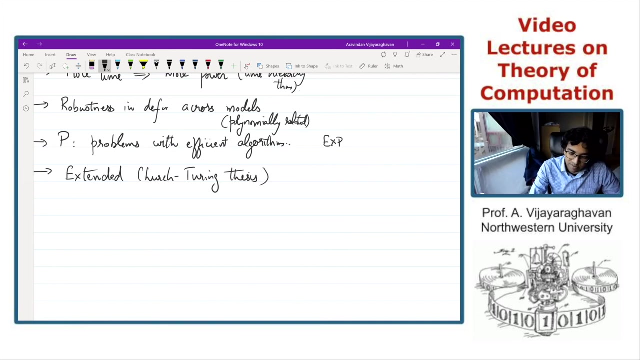 And that's the kind of the in complexity theory. you do care about other classes as well. um, maybe one thing to mention going back is: um, you know, there is uh, uh, for instance, a different class called exp, which is maybe the set of all. um, you know, uh, it's a. 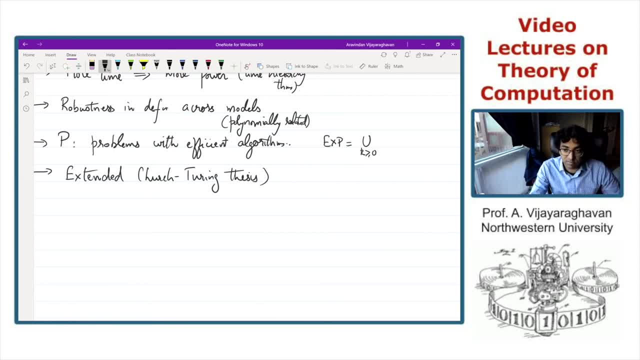 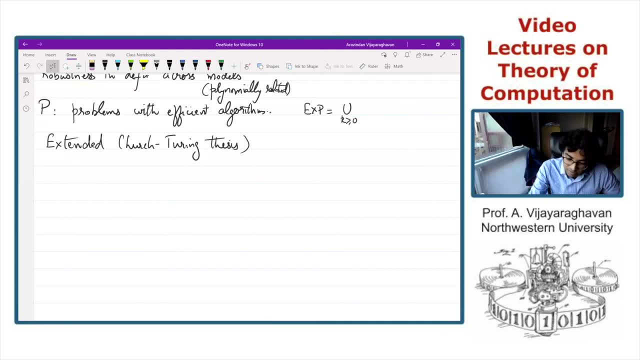 sorry, there was some- which is, for instance, the set of all uh problems for the languages for which you have exponential time algorithms. so this is two to the n, to the k, okay, versus. remember that p is the set of all languages for which you have polynomial time.